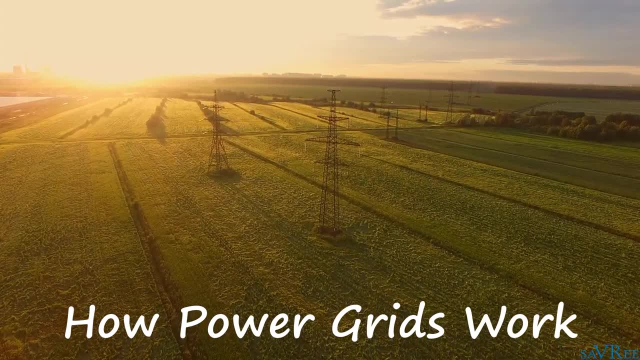 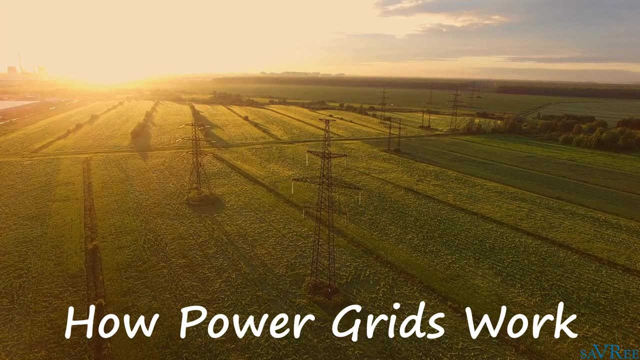 Hi, John, here In this video, we're going to have a look at how power grids work. We'll look at all of the main components that make up a power grid and I'll explain to you how they work together in order that we can get electricity. 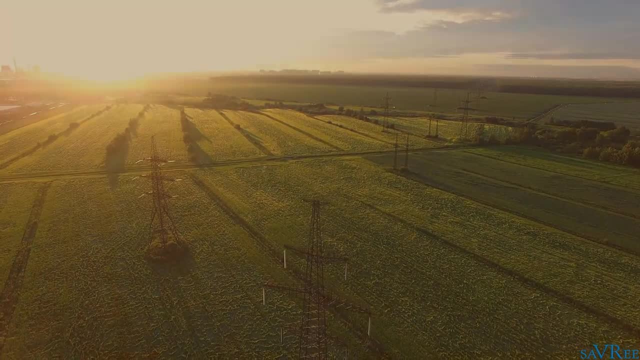 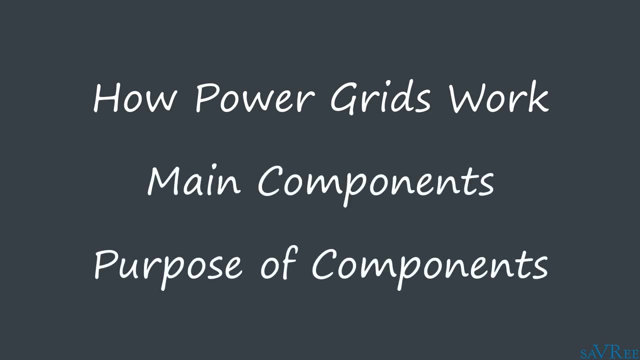 from a power station to your home. By the end of the video, you'll know how power grids work, what all the main components are, what their purpose and function is within the grid and if you're ever out and about in the real world. 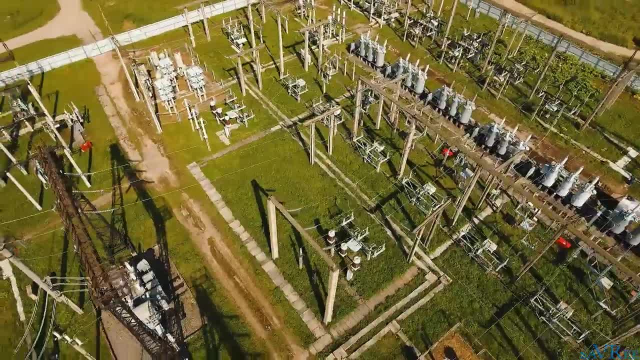 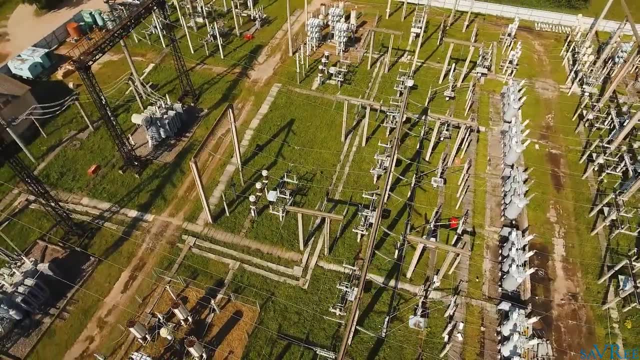 you'll be able to walk past things like electrical transformers or substations or transmission towers, and you'll be able to identify them visually and know why they're there and what their purpose is. So let's start by looking at a basic diagram of a power grid. 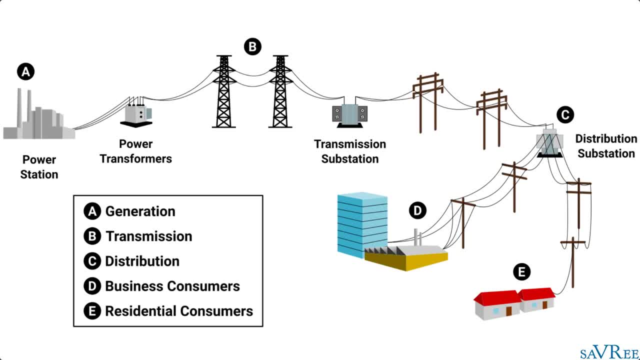 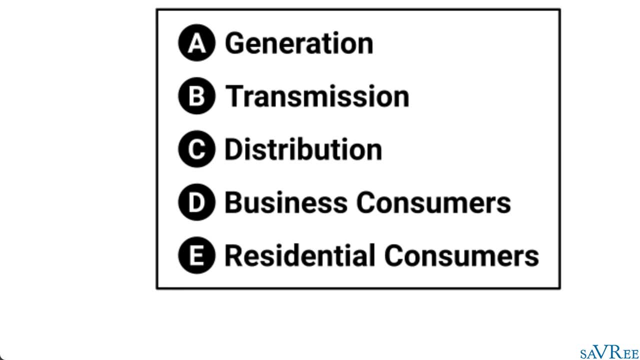 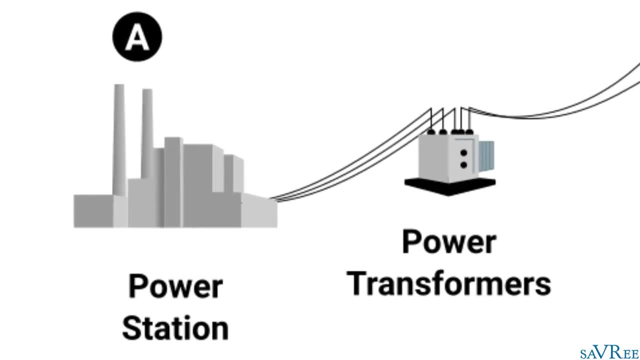 You can see here on our power grid that we've got five letters and these five letters are A, B, C, D, E and they indicate different parts of our power grid. If we look at letter A, it marks the generation part of the power grid. 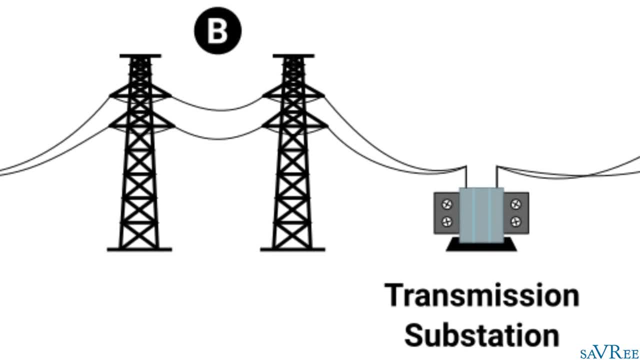 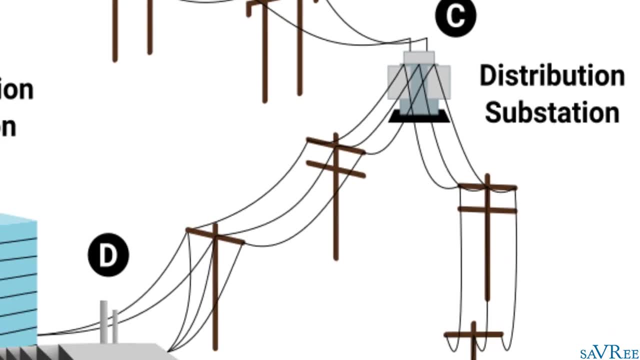 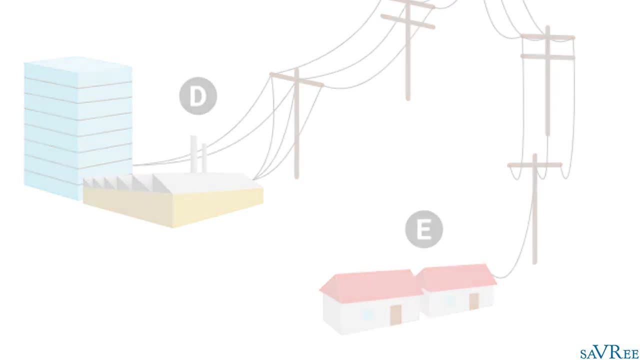 If we look at letter B, this represents the transmission part of the power grid. Letter C is the distribution part, and letters D and E represent our end consumers. Generally, when we're talking about power grids, we split it into three main sections. 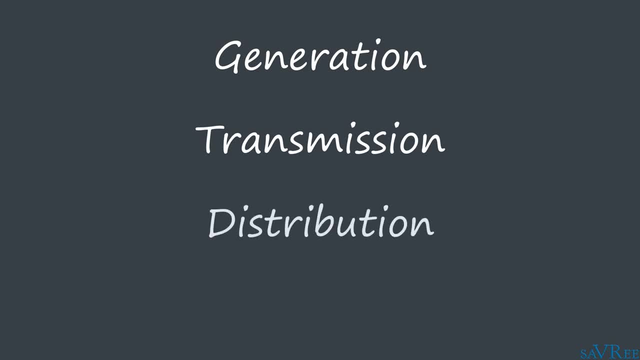 generation, transmission and distribution. If you wanna talk about letters D and E, then we'll simply refer to them as the consumers. I suppose you could call it the consumption part of the power grid. You can see on the diagram that we've actually got some transformers and substations. 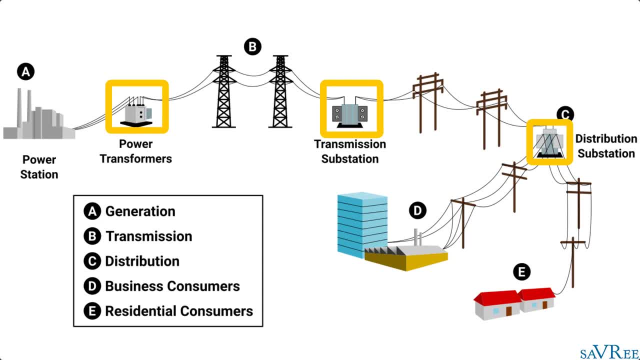 between the letters We've got a power transformer, transmission substation and distribution substation. Don't worry about those too much. now I'm gonna explain to you what transformers are used for and why we have substations, et cetera. 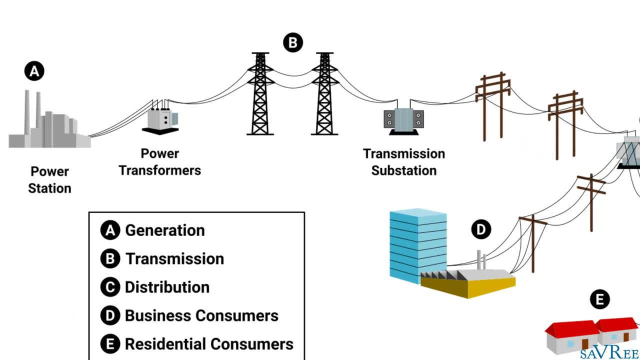 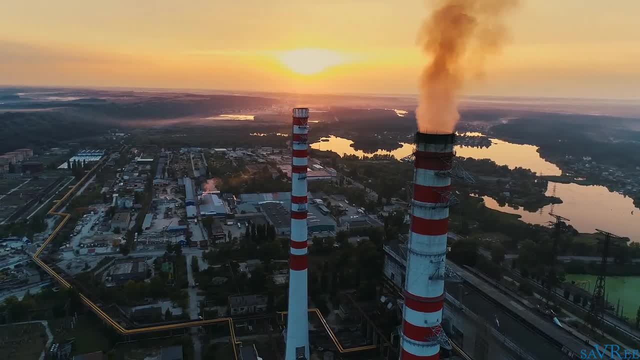 a little bit later in the video. So let's go to letter. A first generation. Now don't be fooled by the name. We refer to it as power generation and the power generation industry, but we're not actually generating any power. 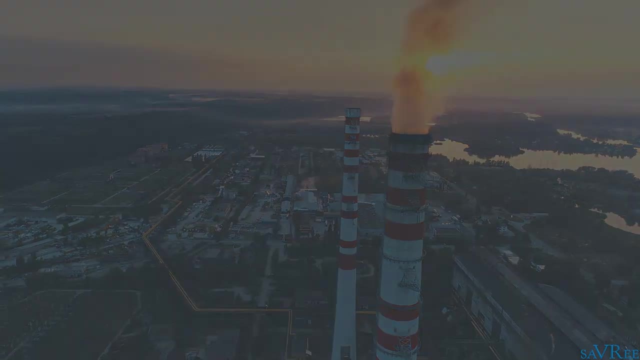 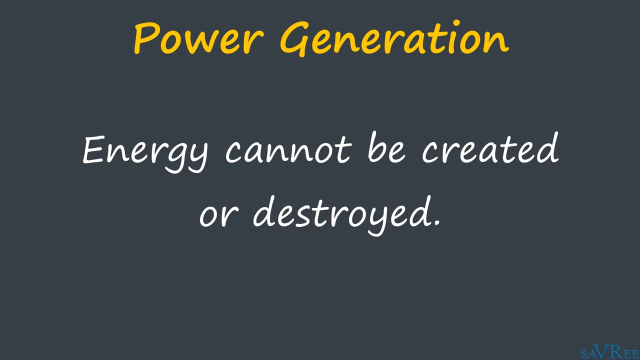 The power that we're referring to is electrical power, and it's not possible to create or destroy energy, and therefore it's not possible to create or destroy electrical power either. If you wanna get technical, this is actually called the first law of thermodynamics. 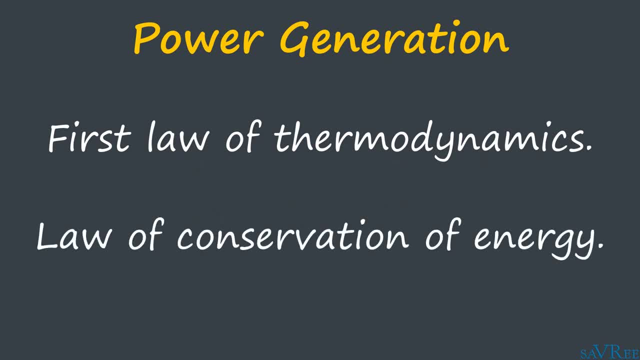 also known as the law of thermodynamics. This is the law of conservation of energy, and it simply means that we can transfer energy from one form to another, but we cannot create or destroy it. So, in order to get the energy that we're gonna put into our power grid, 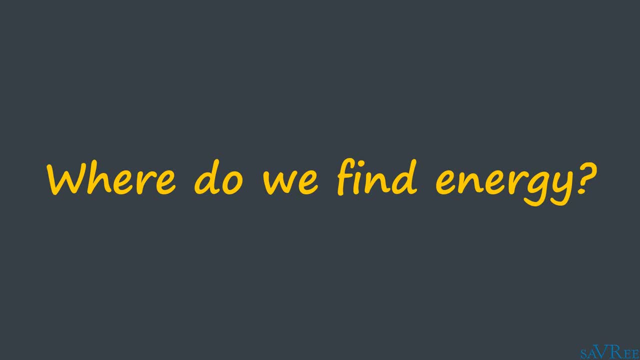 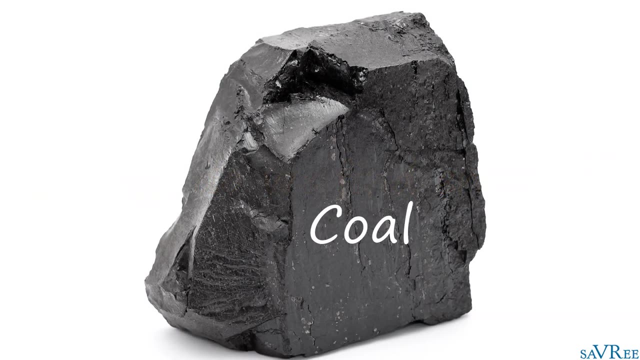 we're going to need to find another energy source and then convert that energy source into electrical power. Now, there are various ways of doing this. If we're burning coal, then we burn coal within a furnace, We release the chemical energy and then we put it in a furnace. 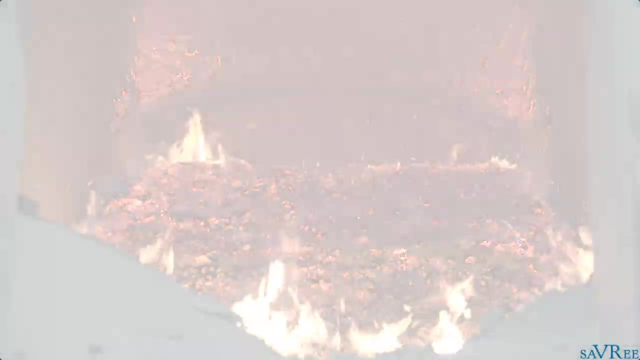 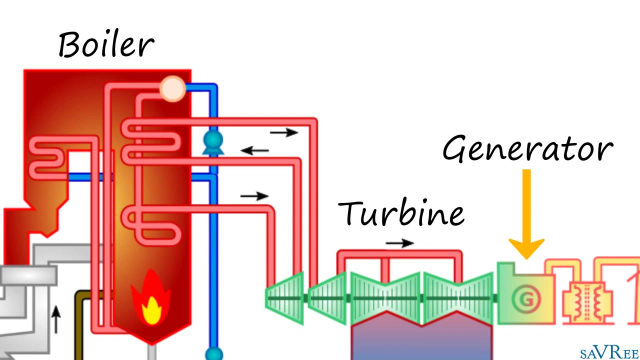 We release the chemical energy that the fuel contains. We turn it into heat. We transfer that heat to water. The water gets heated up and turns to steam. We put the steam through a steam turbine. The turbine rotates and we transfer the mechanical motion. 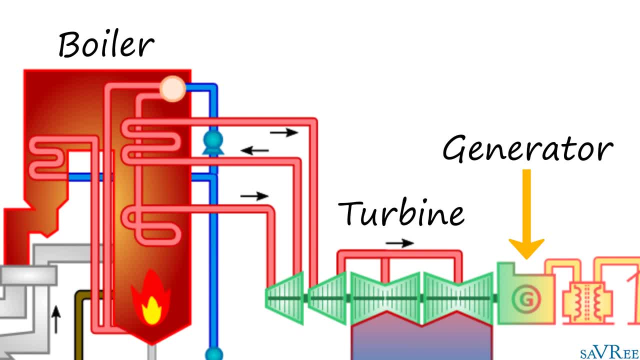 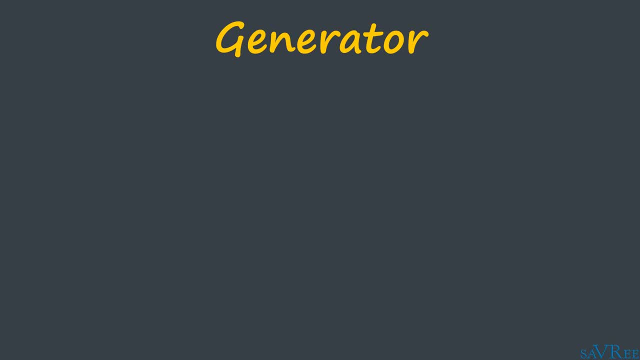 that is, the mechanical energy can also say mechanical power to a generator. Now this generator is actually what they refer to as a synchronous three-phase generator at least 95% of the times in the power industry. and it's actually a three-phase generator at least 95% of the times in the power industry. 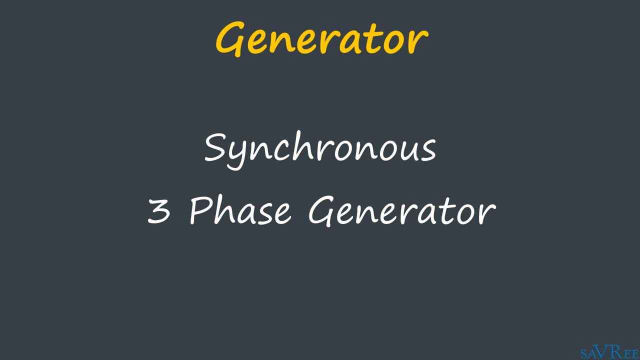 that's what it will be, And the generator converts the mechanical power that it's getting from the steam turbine into electrical power. So we started with chemical energy that's contained within a fuel and we burnt it and we turned it into, in the end, electrical power. 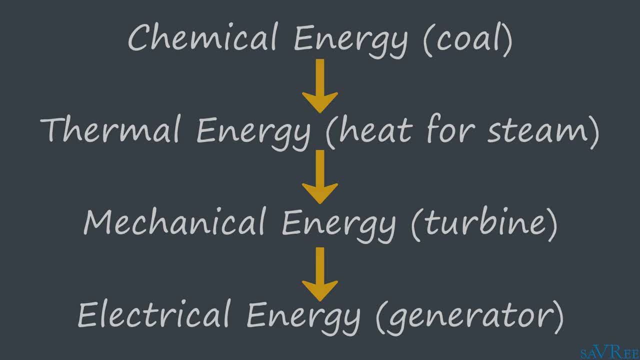 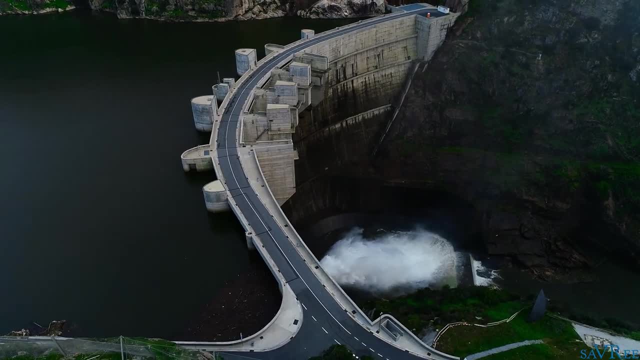 If we're looking at a hydroelectric power station, we'll take the pressure energy or potential energy. we'll take the kinetic energy and we'll harness this by letting it flow across a hydro turbine runner. The runner rotates and then we pass this mechanical motion. 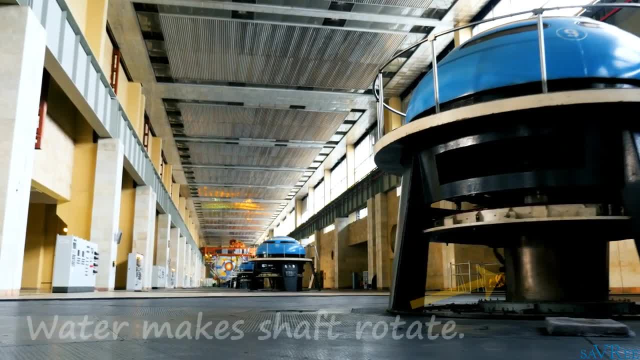 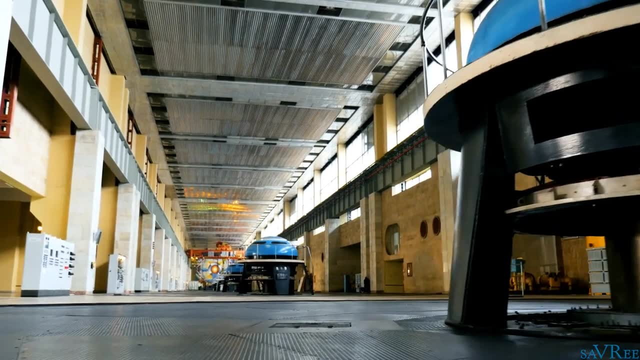 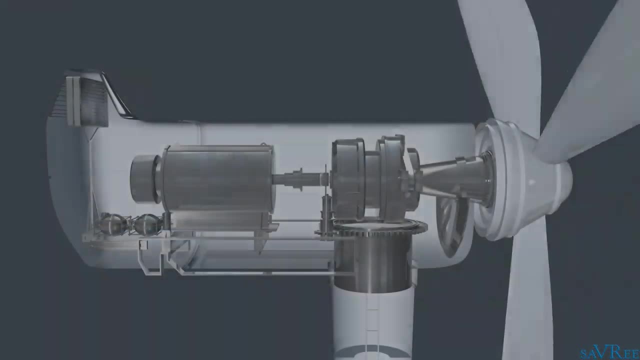 or mechanical power onto our generator and the generator turns that mechanical power into electrical power. So there are a number of different ways in order that we can harness different energy sources in order to get our electrical power. Those are just two common ones. 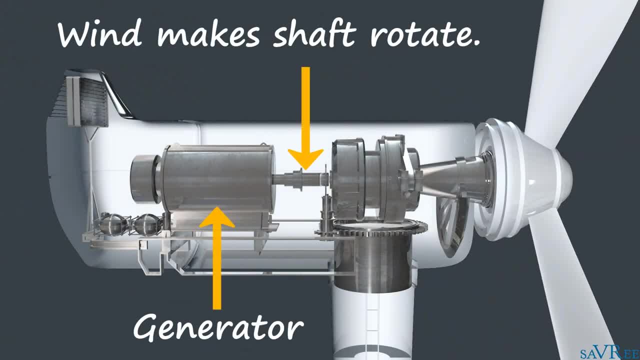 A wind turbine is much the same. We're just taking rotary motion and using that to rotate a rotor in a generator. So now that we've generated our electrical power- I say generated, but I suppose we really should say converted- Either way, we've got our generated electrical power. 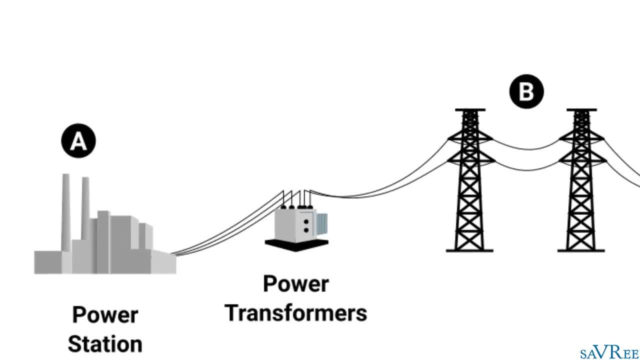 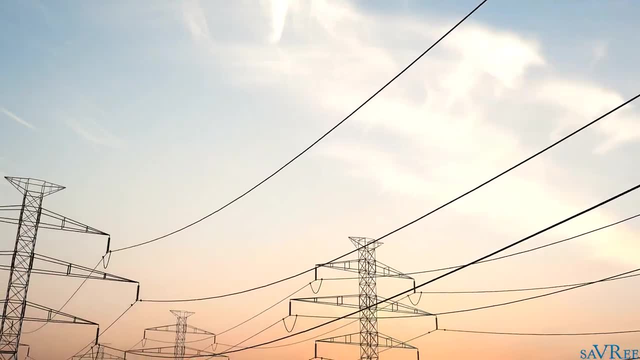 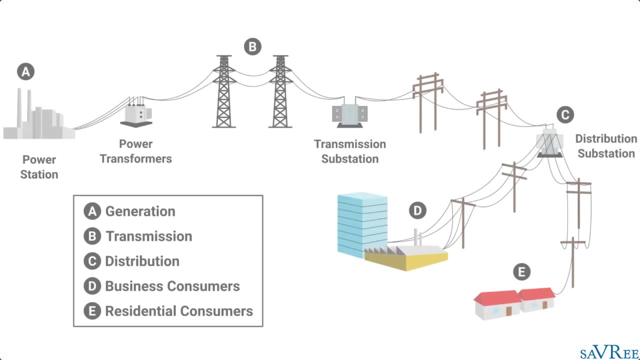 and now we're going to need to feed it into the grid so that we can send it to our consumers. Now it's at this point that we encounter our first problem. Most power stations are very far away from end consumers. If we were to lay a cable or an electrical cable, 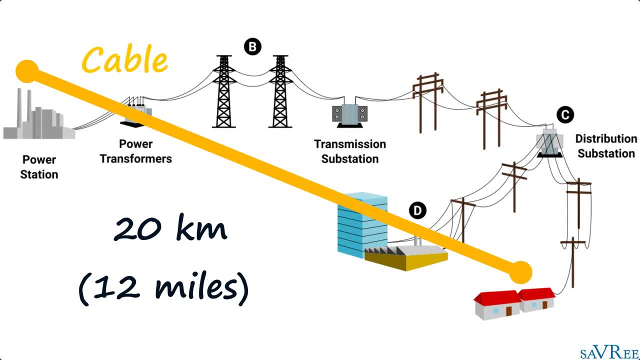 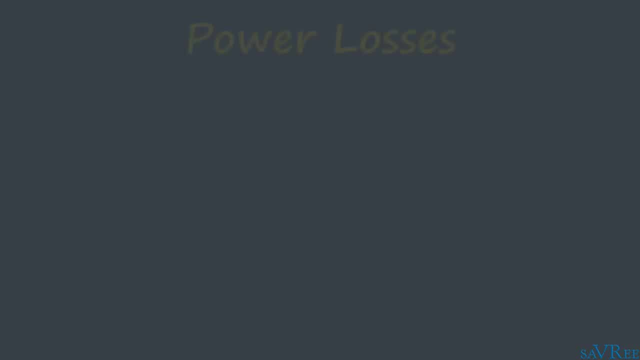 or a conductor, from our power station to our end consumers- and let's just imagine for a moment that our end consumer is 20 kilometers away. well, we're going to encounter losses due to the resistance of our electrical conductor and also due to the heat that's generated. 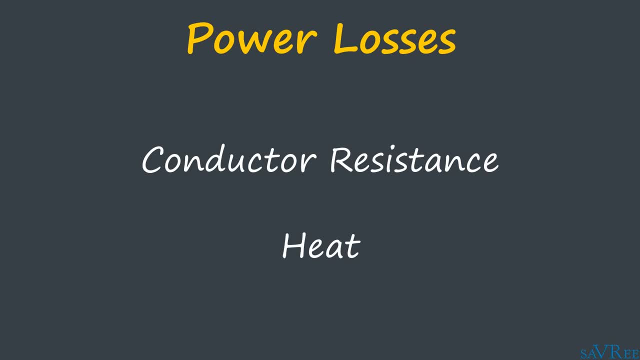 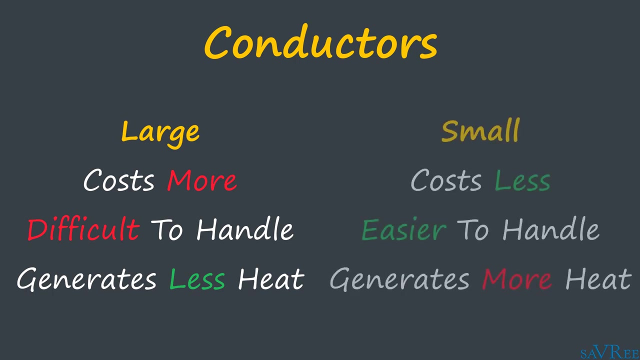 as electricity or electrical current, that is, amps- flows through our conductor. This wouldn't be such a big problem if we could have a very large conductor, but unfortunately, having a very large conductor that stretches across 20 kilometers of land is not very practical. 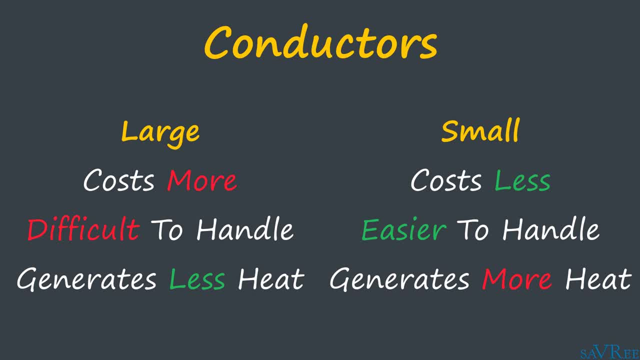 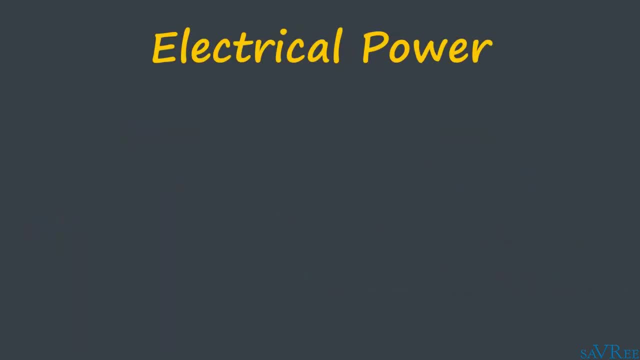 So we need to go back and have a look at why we've got such large losses whenever we dispatch power over a distance. Well, the equation for electrical power is voltage times, current, and the equation for power loss is I squared R: The I indicates current and the R indicates resistance. 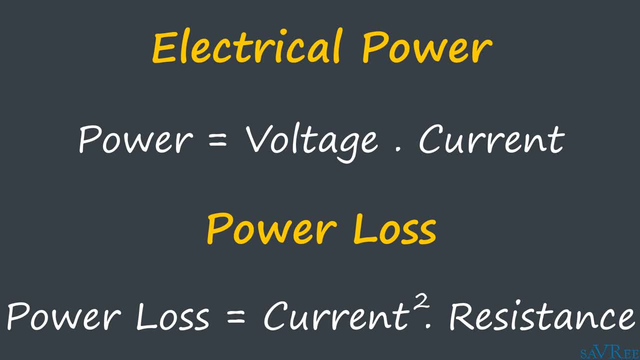 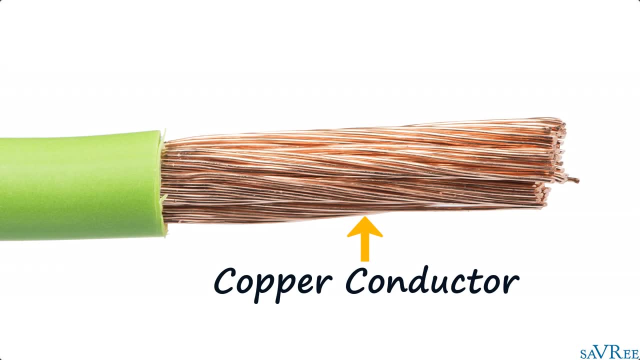 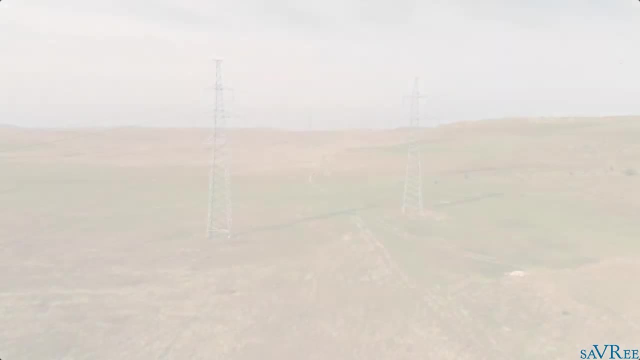 We can vary the resistance in our cables by having good electrical conductors, and these include materials like copper and aluminum, which have high conductivity. But these materials cost a lot of money and considering we're potentially going to need thousands of kilometers or thousands of miles of conductor. 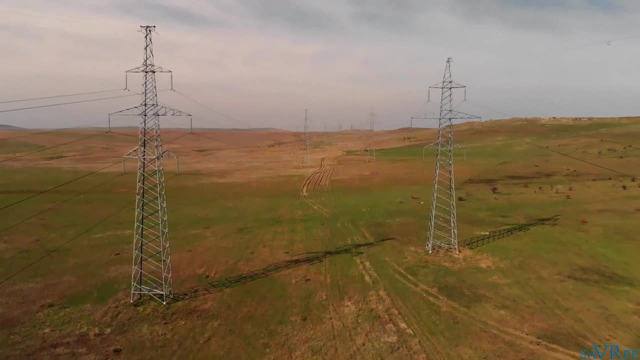 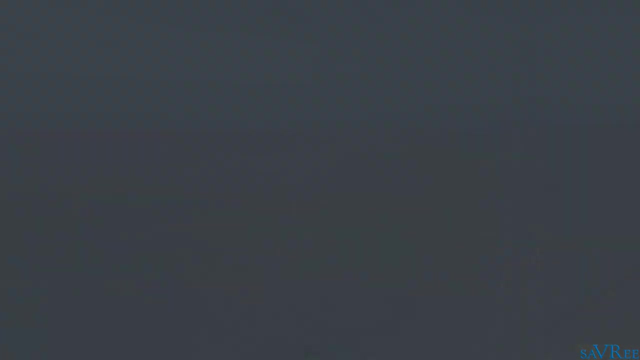 we want to make these conductors as thin as possible, so they need to have quite a small diameter. The problem here is: as we reduce the diameter of a conductor, its ability to carry current reduces. also, When current flows, it generates heat. 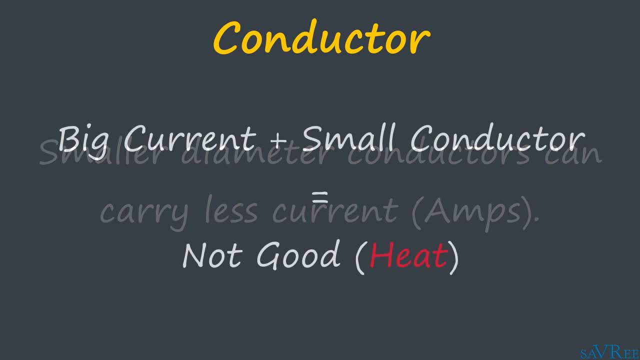 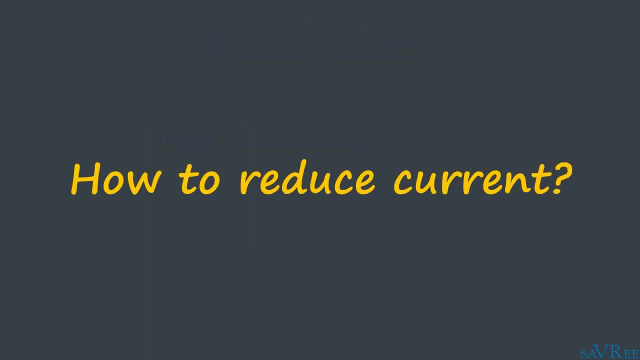 If we have a very thin conductor and a very high current, the current will simply melt the conductor. So how do we reduce the current? Well, we can reduce the current by increasing the voltage. Power equals voltage times current, or P equals V multiplied by I. 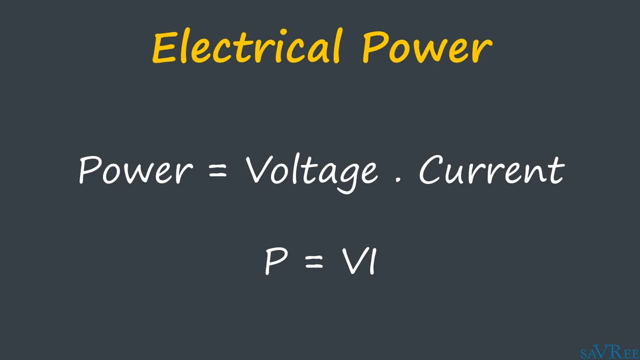 So if we increase V by a factor of 10, then I has to reduce by a factor of 10.. That has to occur because if we want to balance both sides of the equation, the power out has to remain always the same. That means if we increase the voltage, 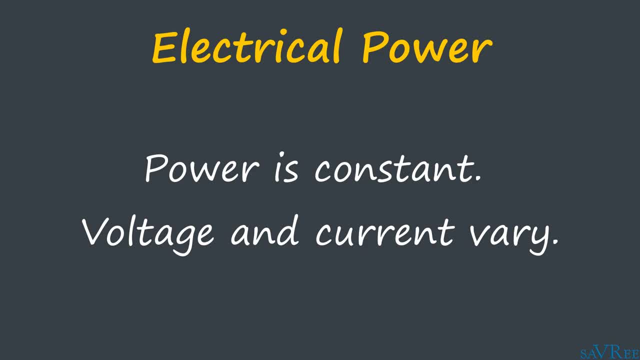 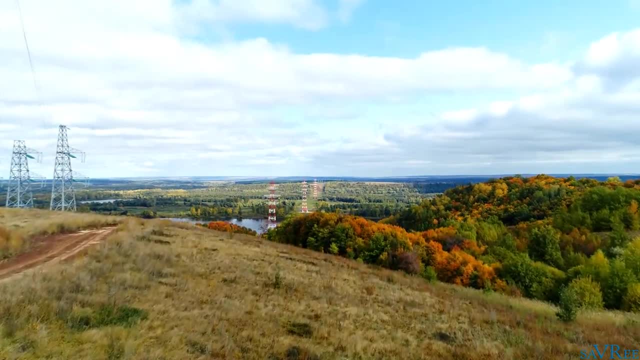 we have to proportionally decrease the current, So we need to increase the voltage. That much we know. And if we can do that, we'll reduce the amount of heat that's generated as current flows through our conductor. That means we can have: 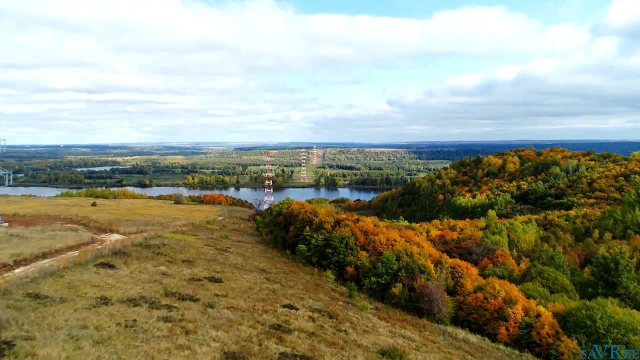 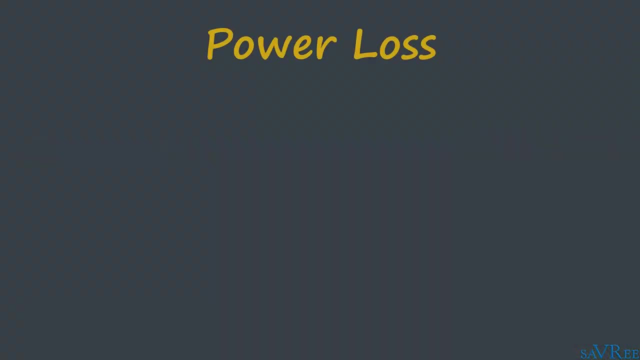 thinner or smaller diameter conductors, which is ultimately going to save us some money. But the other large benefit here is that power losses are represented by: P equals current squared multiplied by R. So power loss equals current squared multiplied by resistance. So the big number here is current. 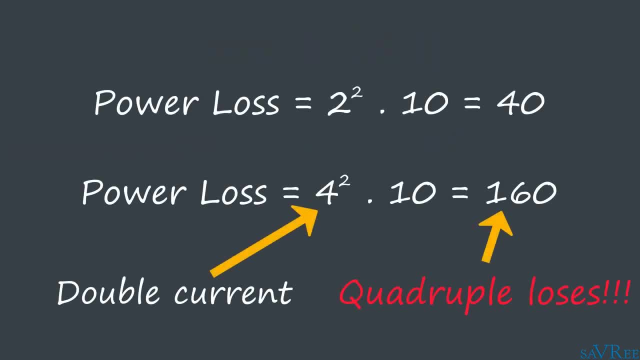 On this example. here you can see that if we double the current and make no other changes to the equation, we quadruple our power losses. That doesn't happen if we double our resistance value. So our priority if we want to reduce power losses. 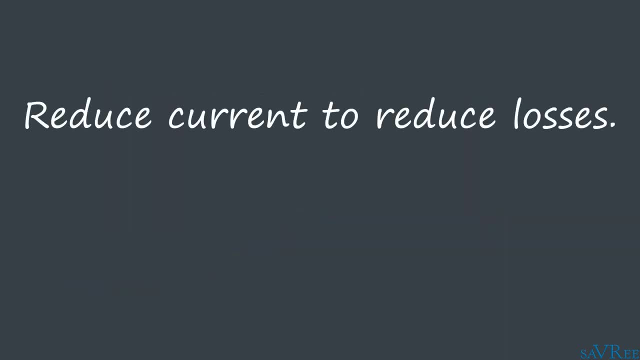 is to reduce the value of current, And we can do this by increasing the voltage. So, to recap, in order to have smaller conductors, which ultimately saves us money because they can be much thinner or have smaller diameters than larger conductors. 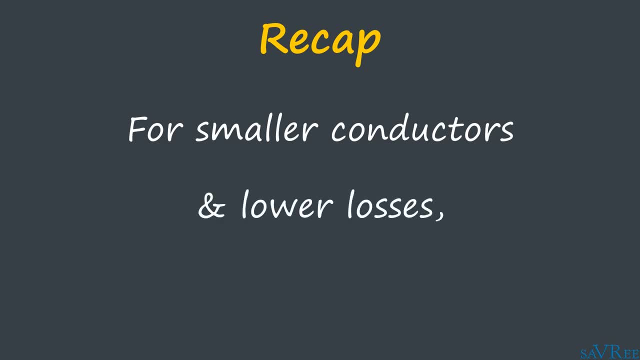 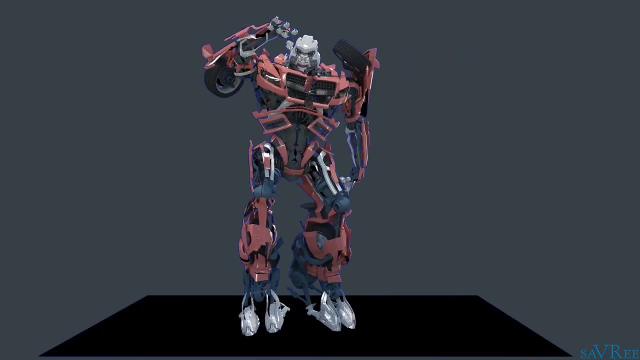 and in order to reduce our power losses, mostly due to the generation of heat, we need to reduce our current level as much as possible. How are we going to do that? This is why we have electrical transformers. People underestimate just how important electrical transformers are to our daily lives. 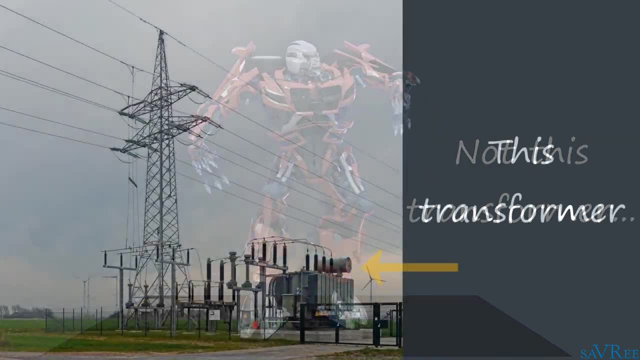 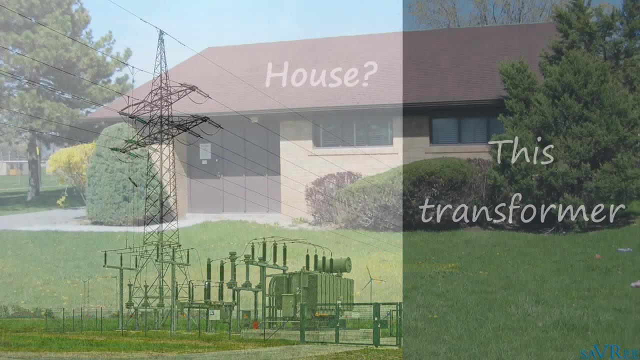 You may think that they're not that important and perhaps you may think you haven't seen many of them around before, But if you live in a city or town, I can guarantee that there'll be a change. but there'll be a transformer within about 400 meters radius. 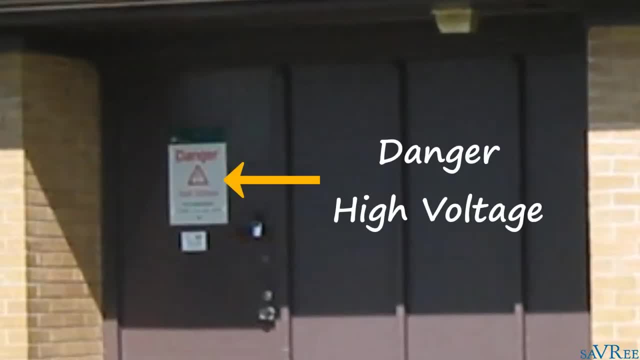 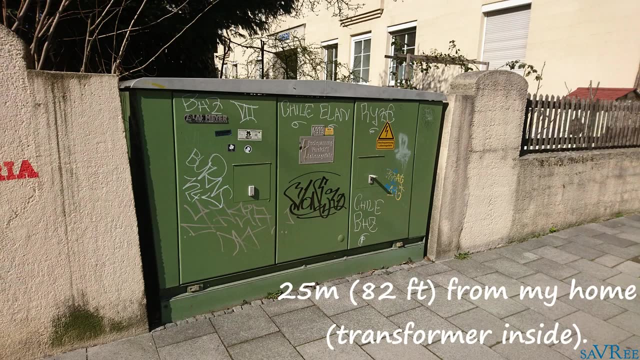 of where you're sitting right now. You might not notice them, because sometimes they're hidden inside houses or small buildings, or sometimes they've just got a wall around them so no one can see them. But they are 100% there. They're essential to the way we live our daily lives. 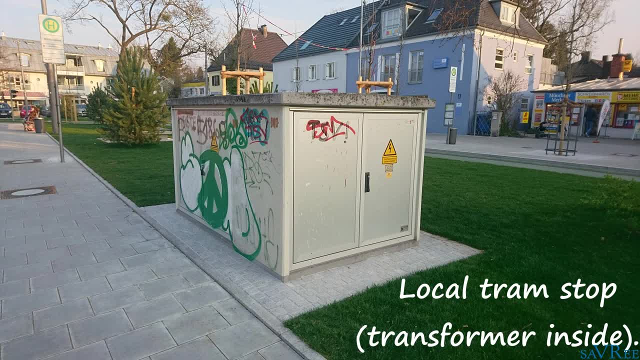 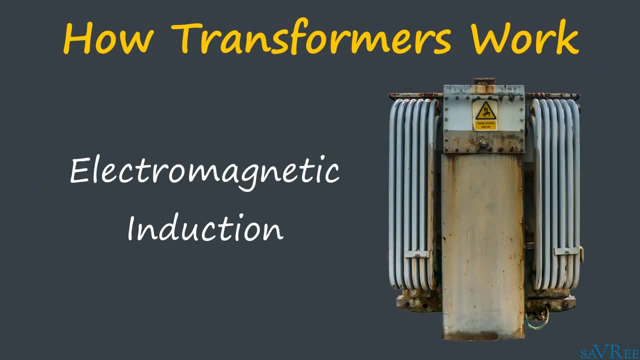 Let's now discover exactly why We need to increase the voltage. We know that much because we need to reduce the current. Transformers work on the principle of electricity Electromagnetic induction, And this states that every conductor that has current flowing through it. 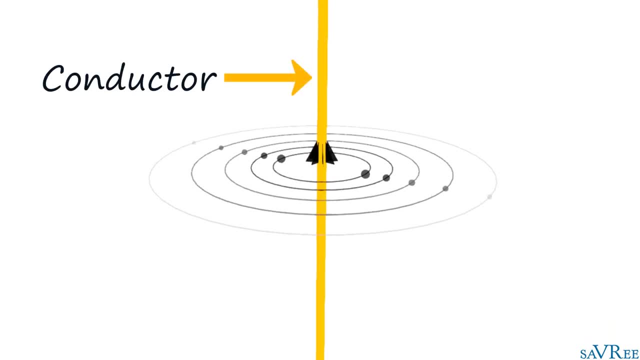 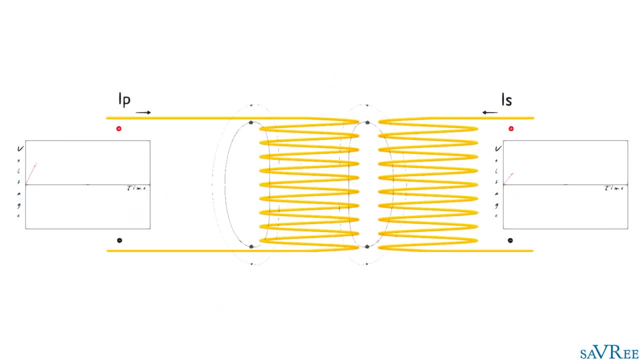 creates a magnetic field. If we take a conductor and we wrap it into the shape of a coil and then we take another conductor and place it nearby, we can actually transfer current from one conductor to the other without them ever physically coming into contact with each other. 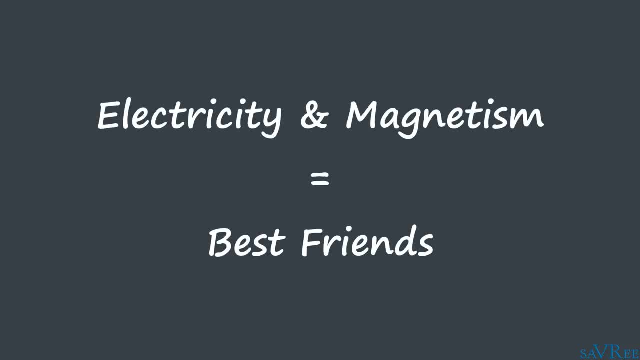 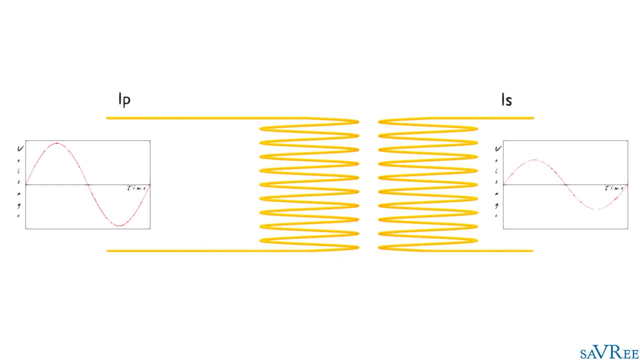 Electricity and magnetism are linked. That means if one of the conductors is connected to a power source, an electrical current is flowing. the magnetic field that surrounds that coil is going to have an impact on the other coil nearby. What's really interesting, though, is this only works with alternating current. 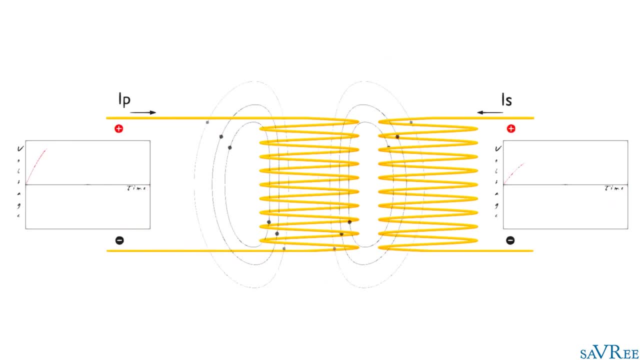 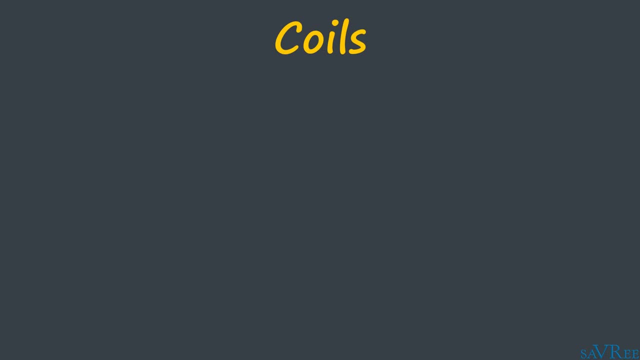 The magnetic field has to be constantly changing in order that we can induce voltage in our other coil. The coil that's connected to the main power supply is referred to as our primary coil. The alternating current that is flowing through that coil creates a magnetic field that expands and contracts. 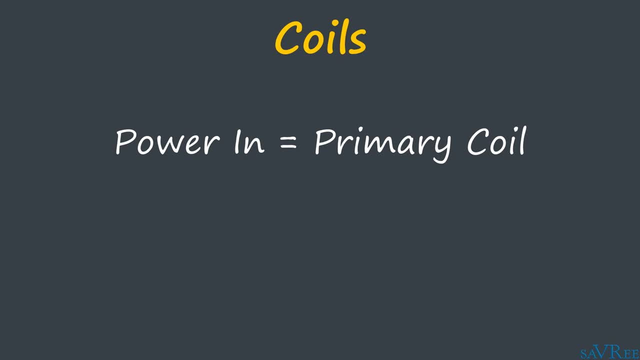 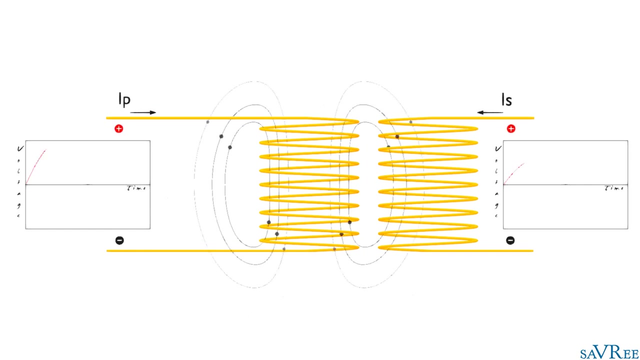 as the current flows back and forth through the coil, This induces voltage in our secondary coil. In this way, we can transfer current from our primary coil to our secondary coil without them ever coming into contact with each other, As current flows back and forth on our primary coil. 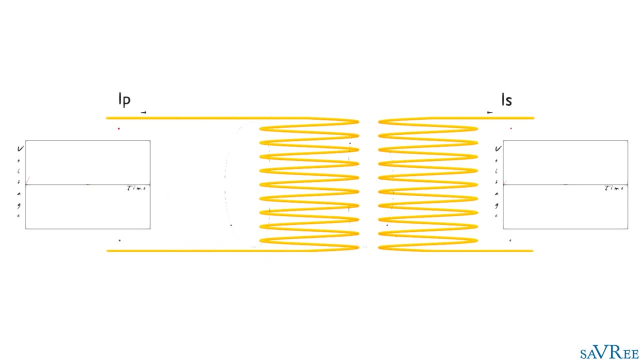 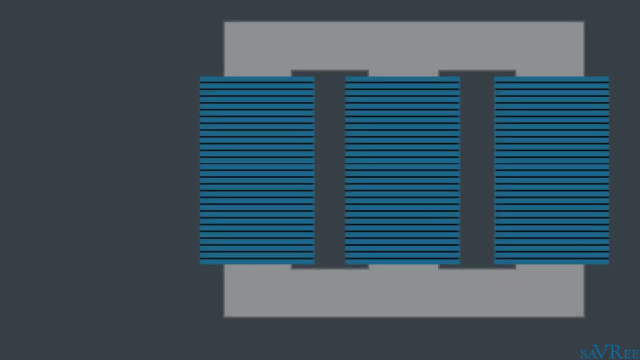 the magnetic field increases and decreases and that causes current to flow back and forth. in our secondary coil In electrical transformers, we actually mount these coils onto a big block of steel. The big block is called the transformer core and although it looks like a solid piece of metal, 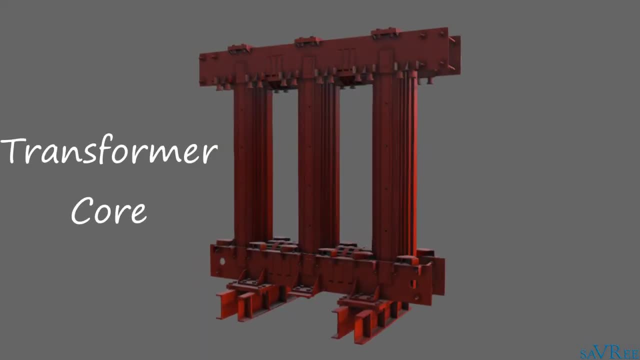 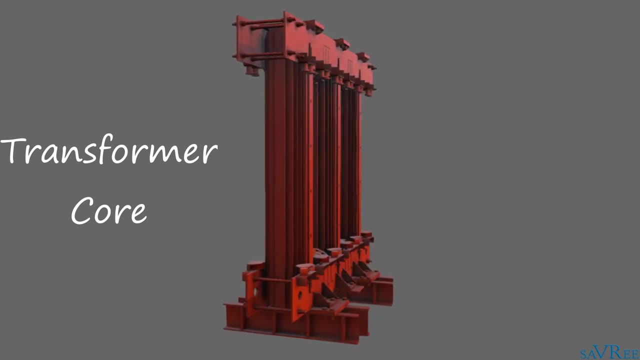 it's actually made up of a lot of thin laminate sheets which are either glued or clamped together. The reason we have the core is just to focus the magnetic field from the primary winding to the secondary winding. The core makes the transformer a lot more efficient. 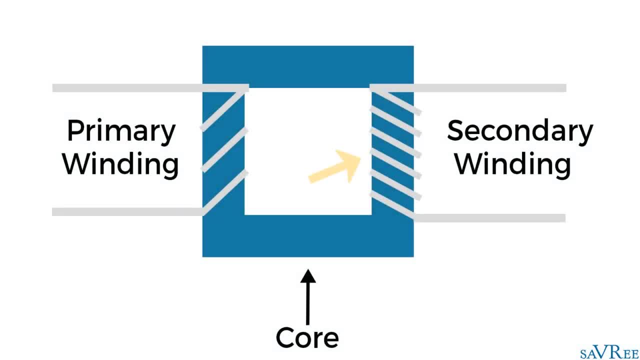 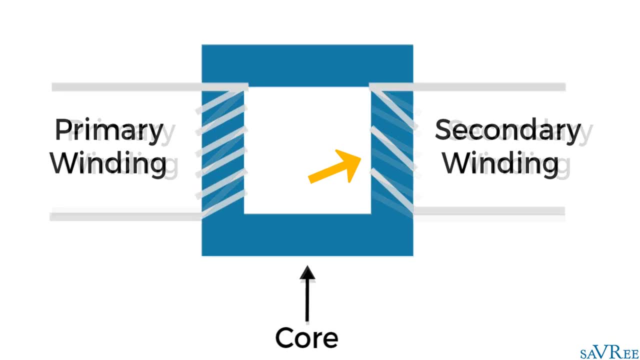 What's really fascinating is if we add more windings to the secondary side of our transformer, we can increase the voltage. If we reduce the number of secondary windings on our transformer, we reduce the voltage. Remember, we want to increase the voltage. 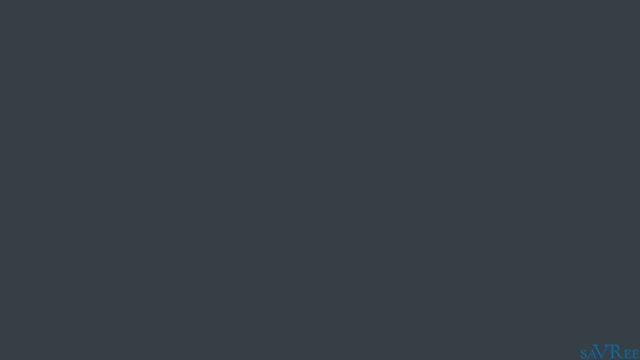 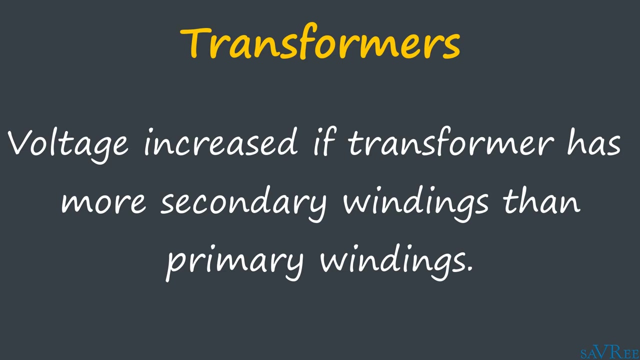 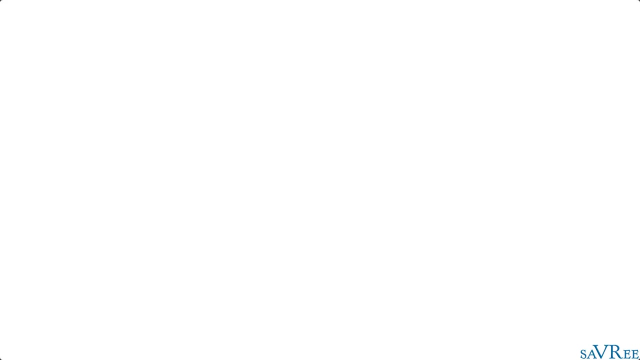 in order that we can reduce the current and reduce our power losses. So transformers that are installed directly after power stations have many, many more secondary windings than primary windings. This allows us to increase the voltage. Transformers that increase voltage are referred to as step-up transformers. 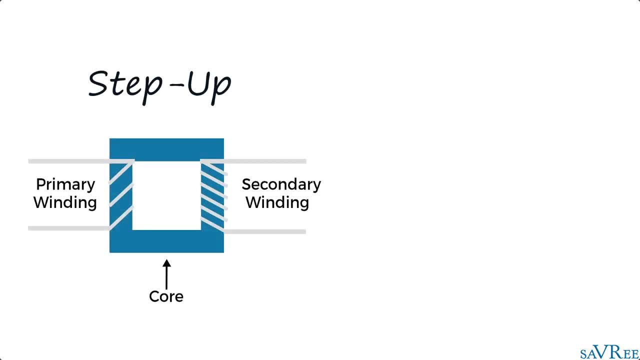 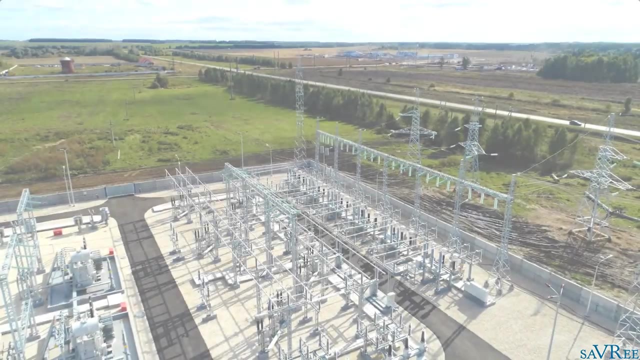 and transformers that reduce voltage are referred to as step-down transformers. The transformer directly after a power station is called a generator step-up transformer, or GSU for short. Once we have increased the voltage, we're going to send our electrical power to a substation. 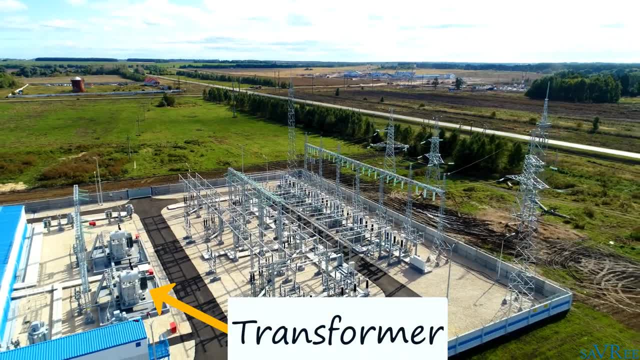 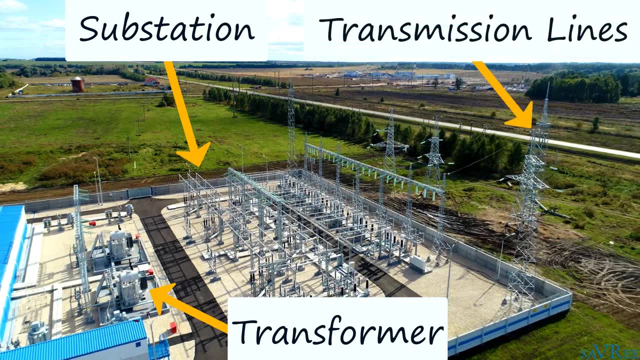 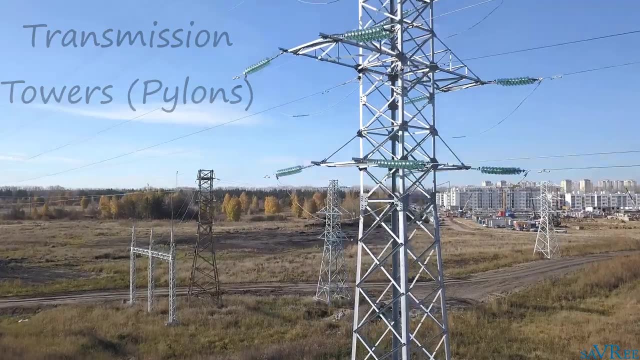 This is usually some type of O2.. This is an open-air switchyard, and then we're going to feed that power into our transmission lines, and these lines are held by our transmission towers. Transmission towers have a very unique shape. They're often very tall, and there's a good reason for this. 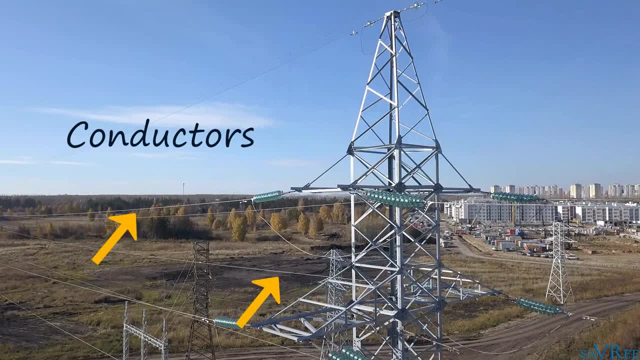 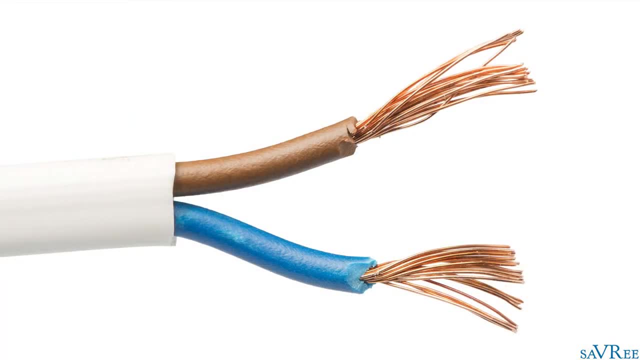 The electrical conductors that are used on our transmission lines are not insulated In your home. when you have an electrical conductor like a copper cable, for example, you're going to have a sheet of plastic or rubber. You're going to have a sheet of rubber around that cable and that is what insulates the cable. 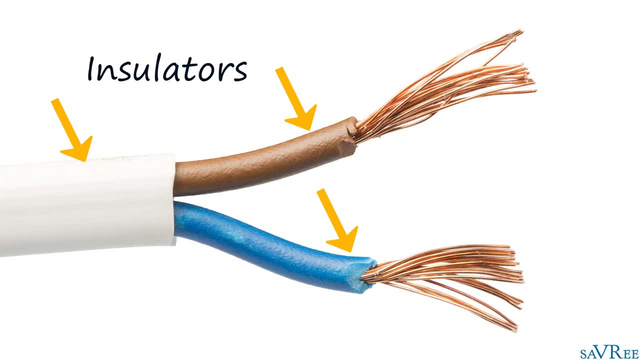 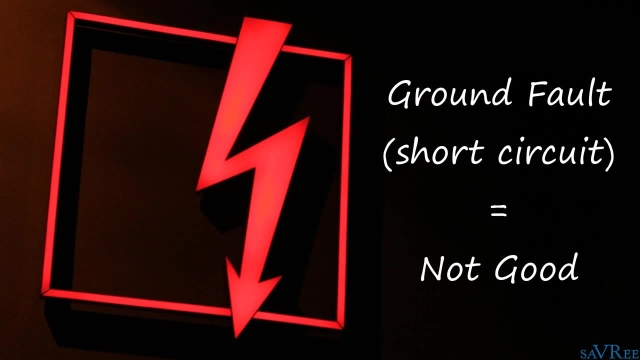 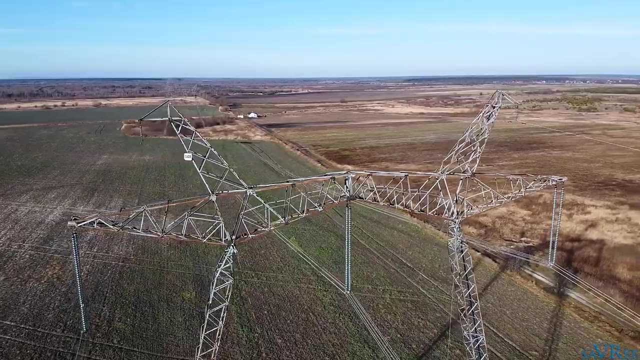 and stops the electrical current from shorting out by going to ground. So we insulate the conductor in our homes in order that current flows where we want it to and that we don't have short circuits. The conductors that we use on our transmission lines do not have any plastic or rubber surrounding them. 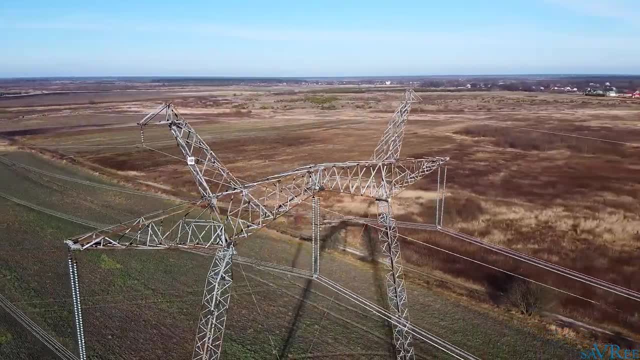 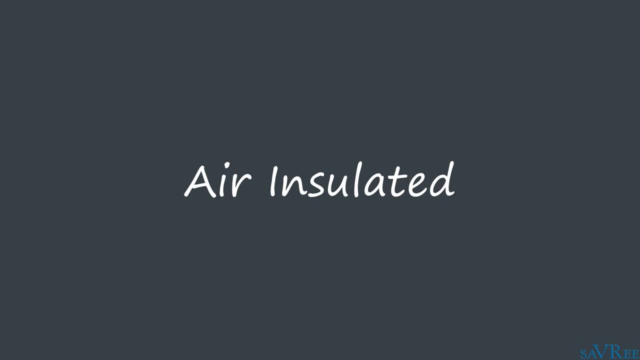 but they are, however, insulated. You just can't see the insulation. They're what we refer to as air insulated, And the reason we have to hang these conductors on a large tower is because air is not such a fantastic insulator that we can leave the conductors hanging around one meter above the ground. 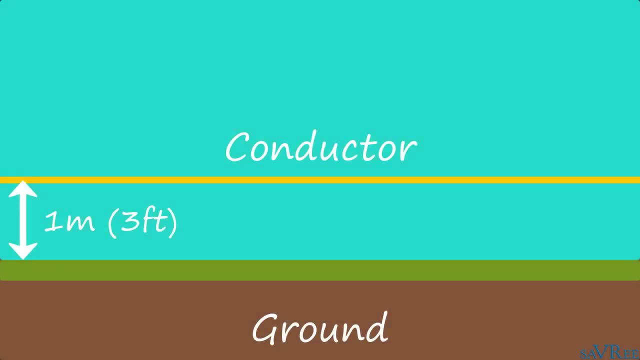 If we did this, the air surrounding the conductor would be ionized to such a degree that we would get an electrical arc from the conductor to ground. This arc would look like a large spark. So we hang our conductors high above the ground so that there is a large 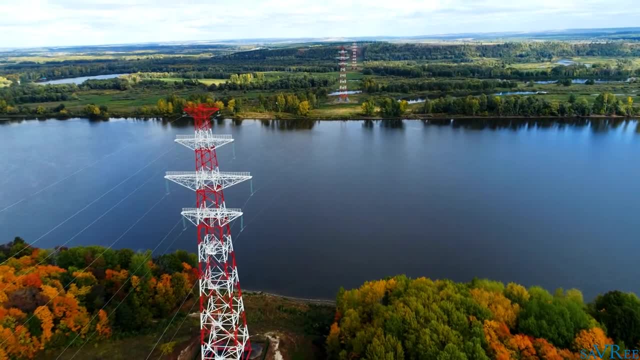 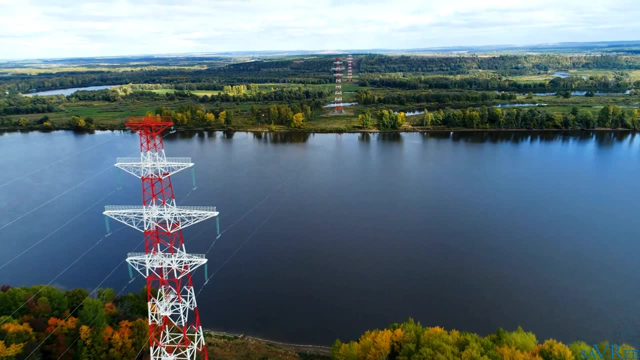 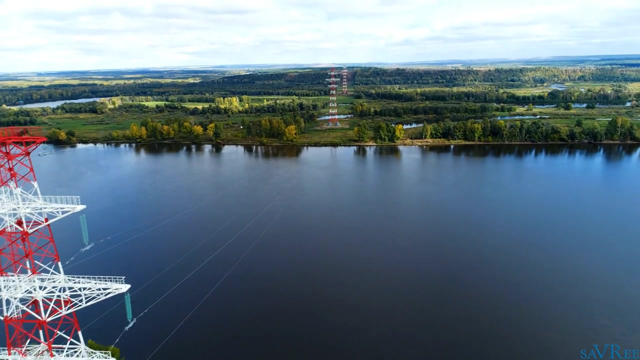 air gap between the conductors and ground. This gives us a large amount of air insulation. Not only that, but it keeps the transmission lines well out of the way of the general public, because we don't want people driving into our transmission lines or accidentally flying a kite into them and causing a ground fault. 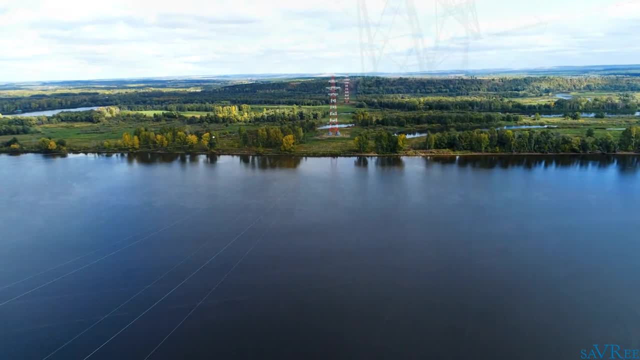 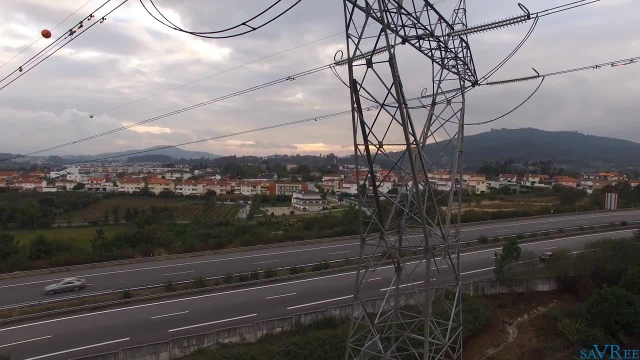 It's not good for the power grid and it's definitely not good for the person holding the kite. Although we've insulated our transmission lines from the ground, we also need to insulate them from the tower itself. This would act as a very efficient conductor if our transmission lines came near. 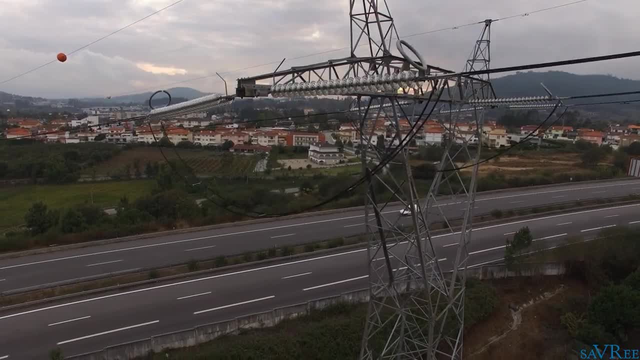 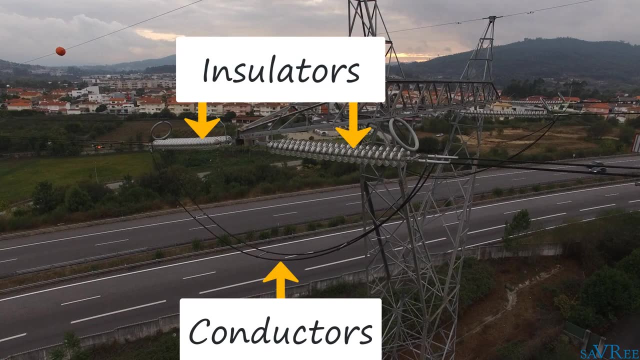 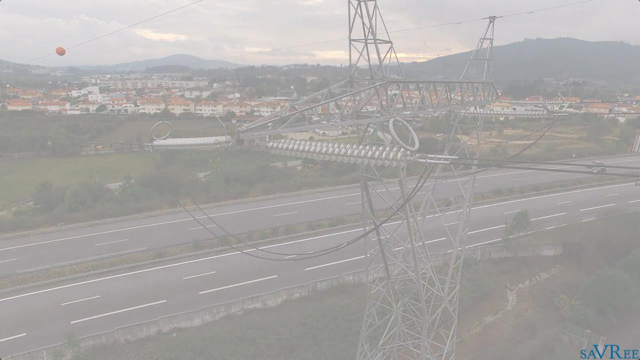 or touched onto the tower itself. To ensure this doesn't happen, we hang our transmission lines from the tower using insulators. Insulators allow us to bring the transmission lines to the tower without bringing them too close to the tower. Initially, when we generated electrical power using our generator. 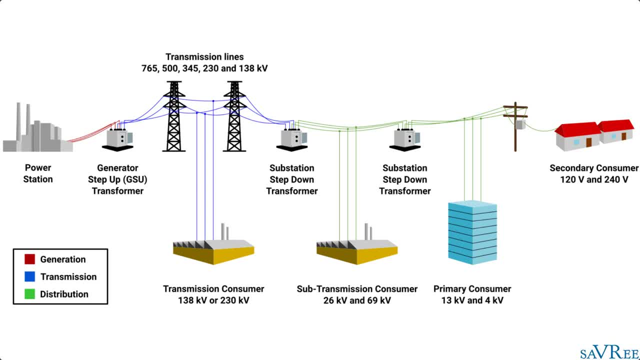 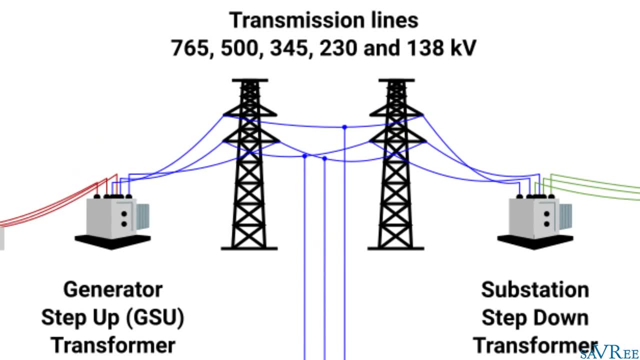 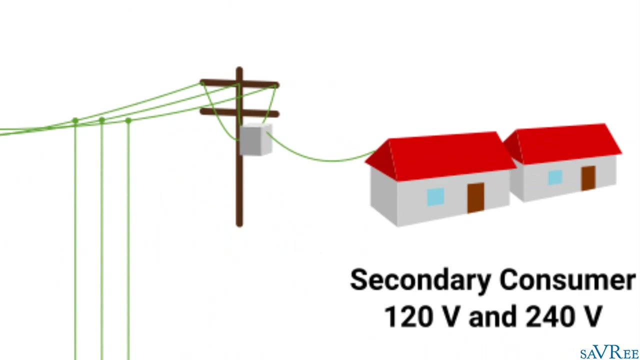 we may have had a voltage of 20 000 volts. When we reach the transmission stage, we may have a voltage of 130, 230, 340, 500 or even 765 000 volts. That is a lot of volts, Especially when you consider in your home you may use 220 volts or 110 volts. 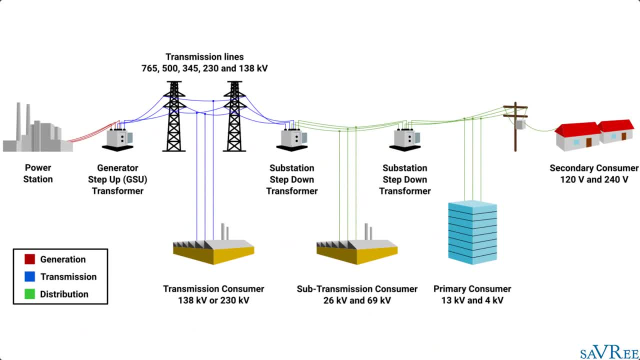 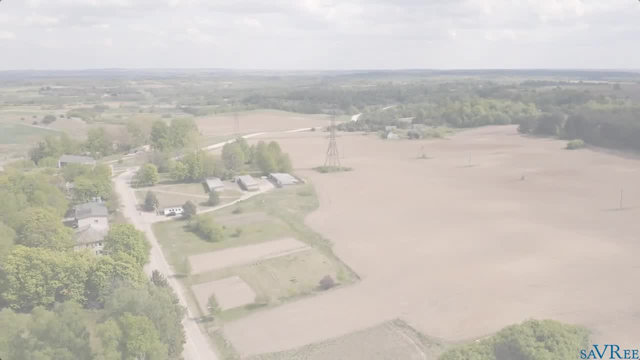 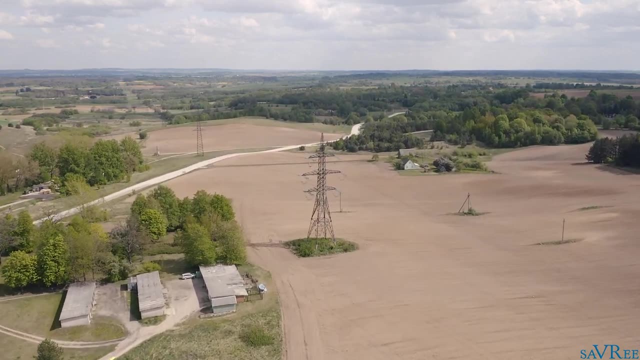 So we've massively increased the voltage in order to reduce our transmission losses and in order to be able to reduce the size of our conductors. We're now distributing our power across potentially hundreds of kilometers or miles before we reach the next part of the power grid. 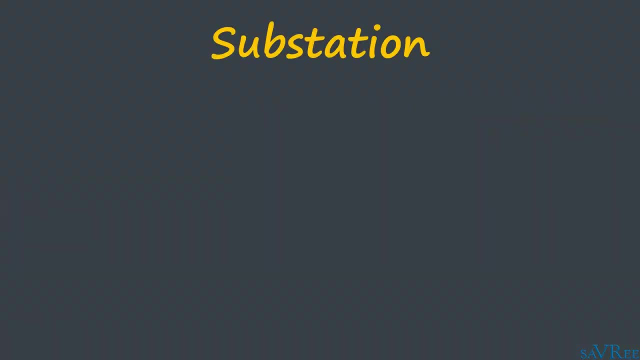 Once again, we reach a substation. Substations contain all of the equipment we need in order to reduce and increase voltage. Not only that, but they allow us to separate various parts of the grid from each other. This means we can protect different parts of the grid from each other. 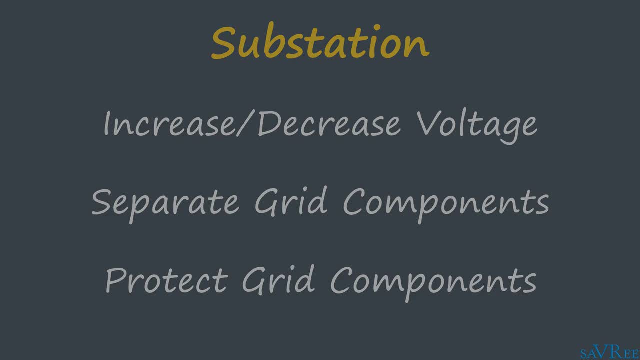 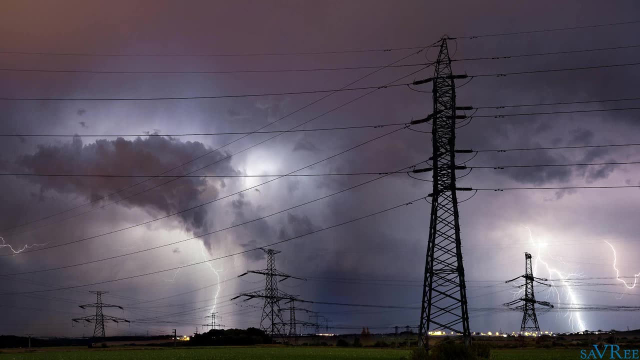 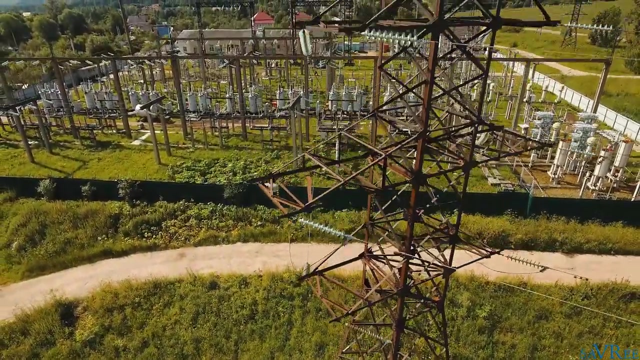 So that if we have things like lightning strikes or power surges, we can isolate certain areas of the grid rather than have a complete blackout. Substations are critical if we want to ensure that the machinery and the components that make up the power grid are as protected as much as possible. 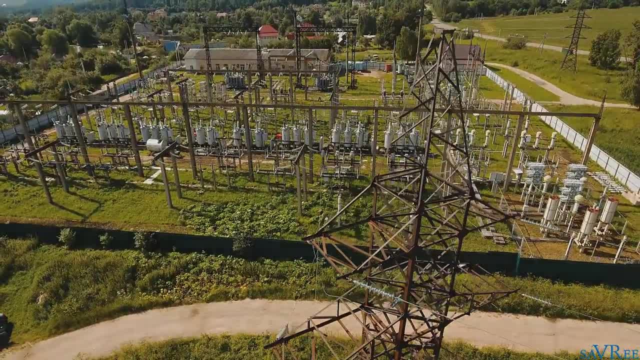 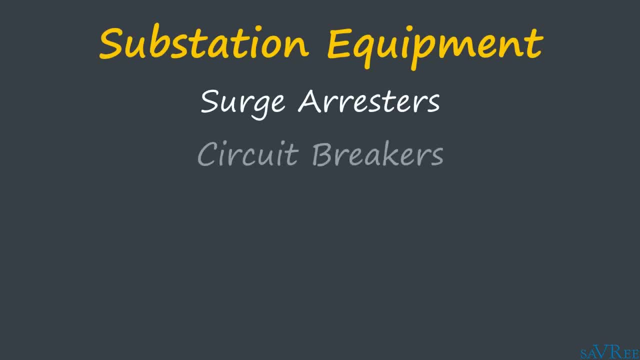 so that we can increase the reliability of the grid. Substations contain items such as surge arresters or lightning arresters, circuit breakers, switch gear, disconnectors and transformers. We've left the transmission stage and now we're going to go to the distribution stage. 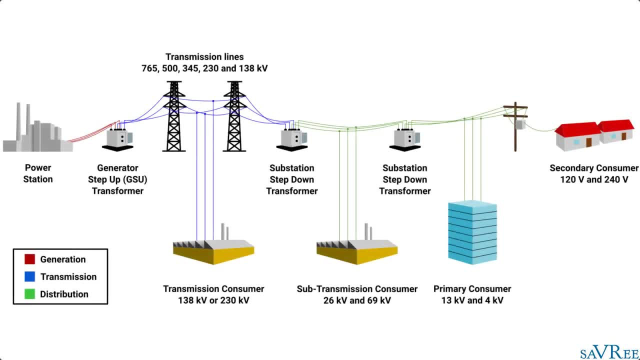 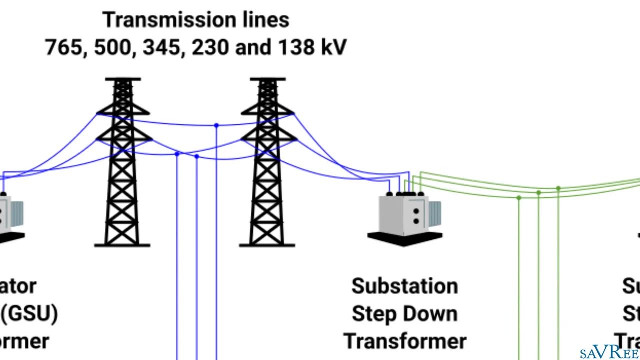 We don't want to send electrical power to our end consumers at 765 000 volts. They're not going to like that very much at all, So we'll reduce the voltage using a step-down transformer. and remember, this is a transformer that has far fewer windings on the secondary side than it does on the primary side. 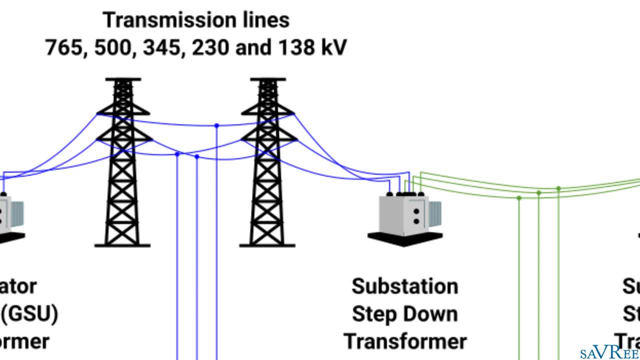 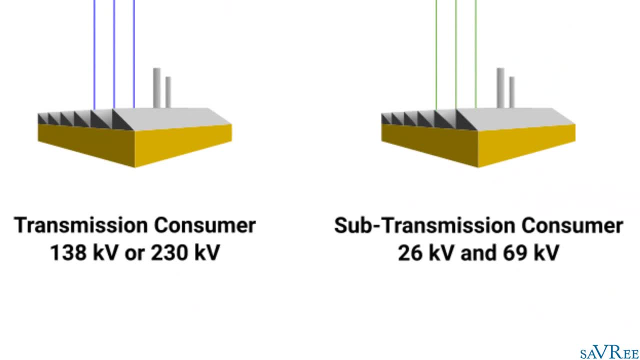 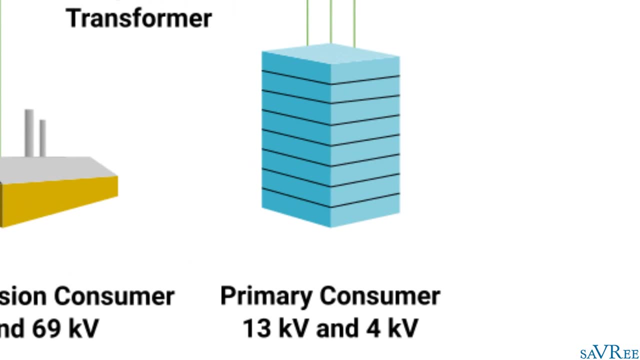 Different consumers require different voltages. Industrial plants, for example, may require voltage to be delivered at 30 000, 20 000 or 10 000 volts, depending upon the application of the plant. Large office buildings and hospitals will require lower voltages, and by the time we reach the 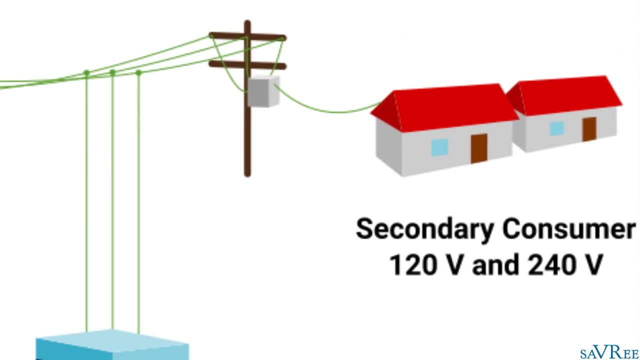 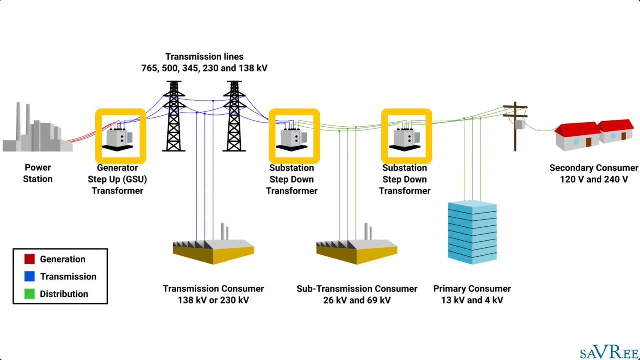 general consumer living at home. they're going to require voltages of 380 volts to 40 volts, or even 110 or 120 volts. Because there are multiple consumers requiring multiple voltage levels, we're going to need multiple transformers and each specific transformer is going to cater for one specific voltage level. 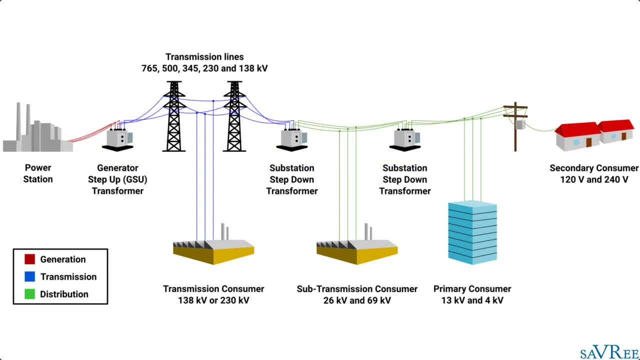 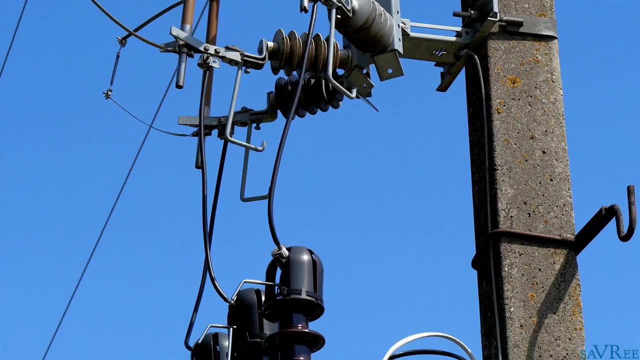 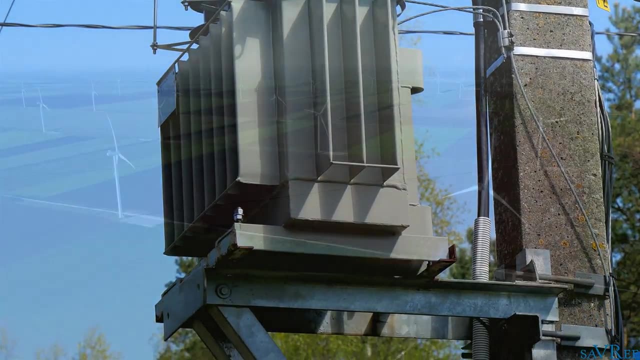 Now that we've reduced the voltage to quite low levels, it's essential that we deliver that electrical power over as short a distance as possible, and this is the reason why, if you're living in a city or town, a transformer will be located nearby. So you now know how we get electrical power from our power generation source. 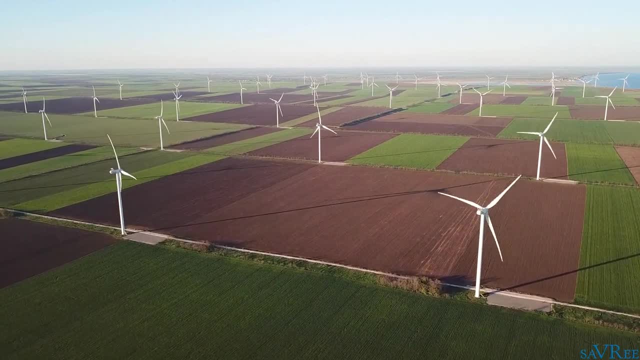 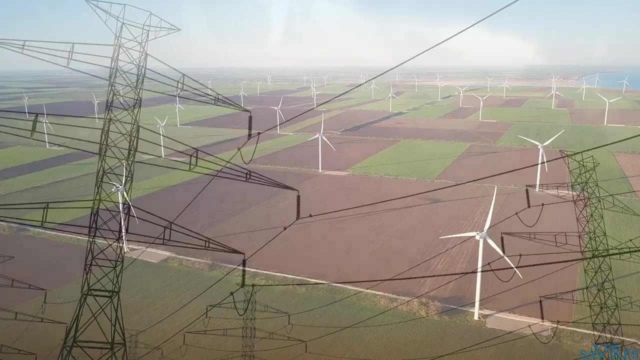 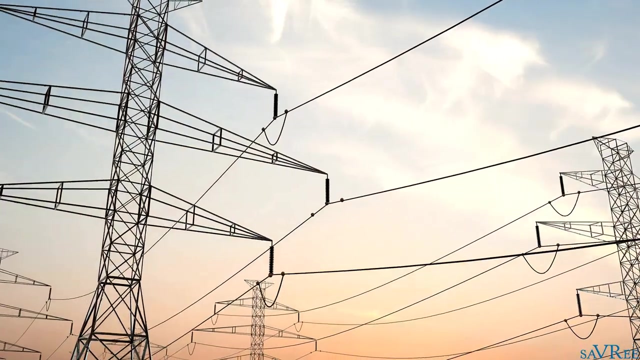 which may be a coal-fired power station, perhaps a series of wind turbines or a hydroelectric power plant, etc. and how we transfer that electrical power to our homes, even though our homes may be miles and miles or kilometers and kilometers away from the power source. If you want to learn more about engineering, then be sure to check out our website. we've got over 25. 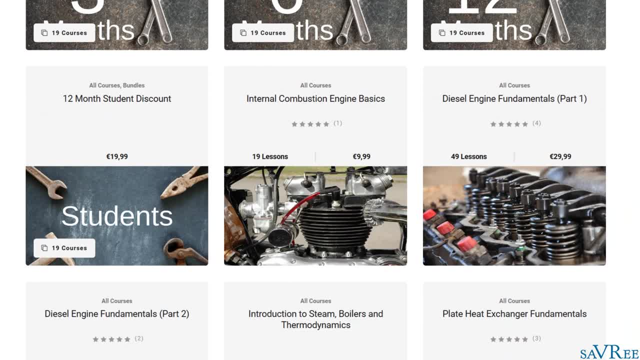 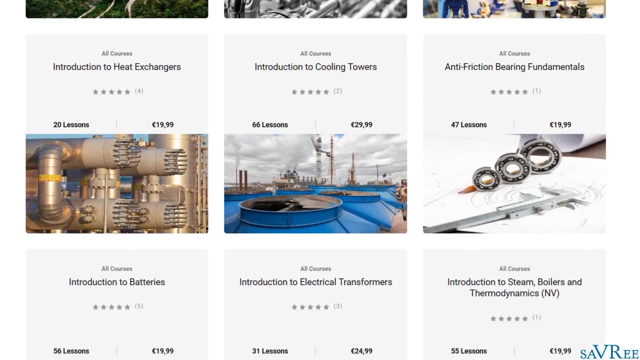 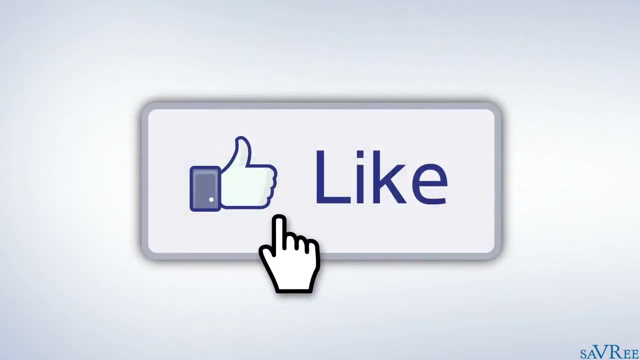 hours of engineering content. We cover everything from diesel engines to valves, to pumps to power stations. If you think that sounds interesting, then check out the links in the video description area. If you enjoyed this video, then please do like it or share it on social media. it really does help us. 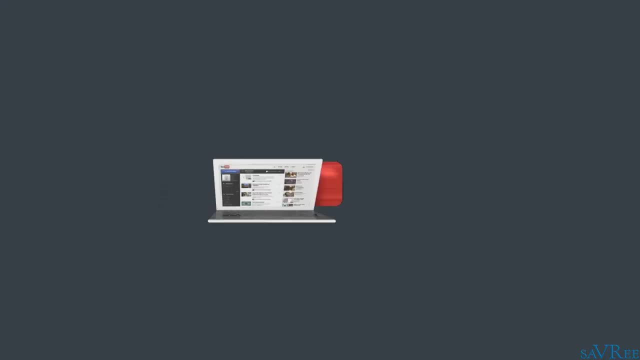 out and don't forget, you can subscribe to the youtube channel. Thanks very much for your time. 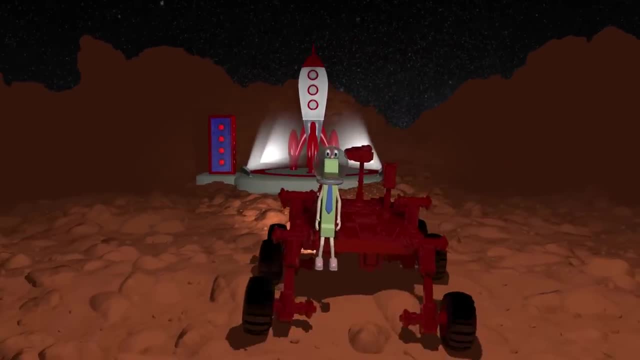 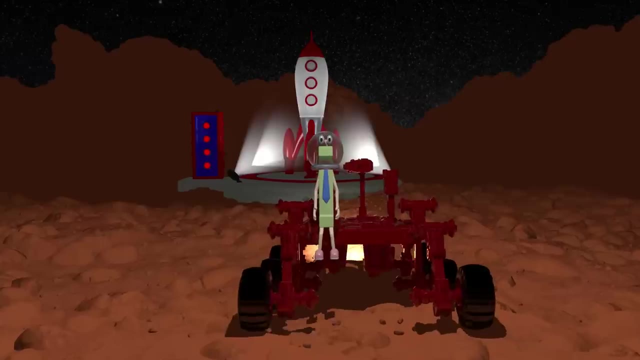 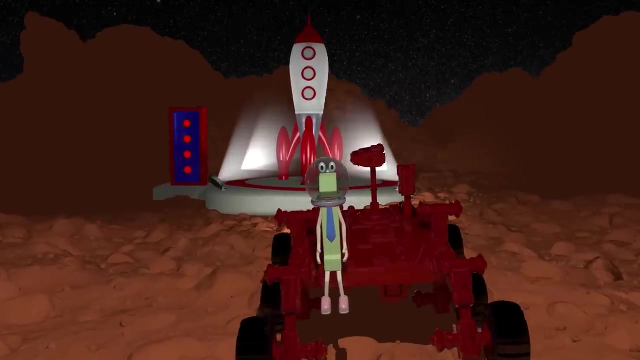 Hey guys and welcome to the Red Planet. I am here hitching a ride headed towards my spaceship to take me home. The only problem I have is that I need fraction power and we are low. You see, my spaceship runs on fraction power and in order to get the batteries full, 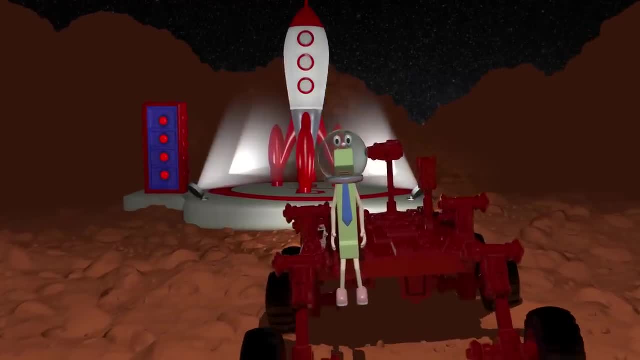 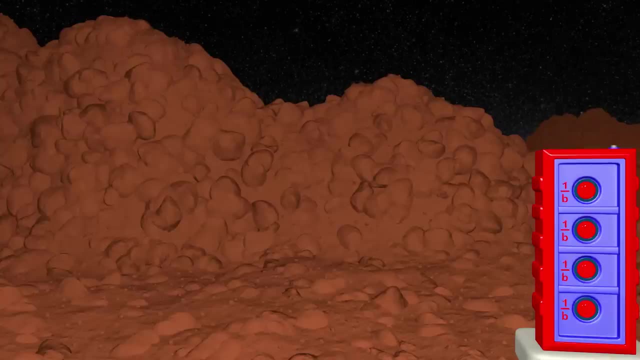 I need to put in the right fractions to recharge the batteries. Let's charge the batteries with the fractions I have collected and then I can go home. Here we are at the charging station. The first thing we need to do is review what is a fraction. 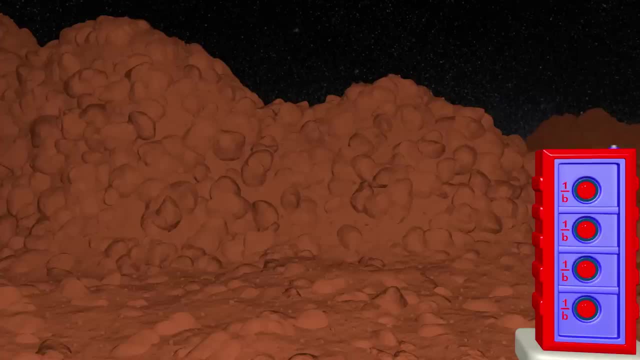 You may remember from my other videos, but just in case you forgot, here we go. A fraction represents an equal part of a whole. Here we see two circles, but only one circle represents a fraction. Can you guess which one? If you guessed the red circle on the left, you are right. 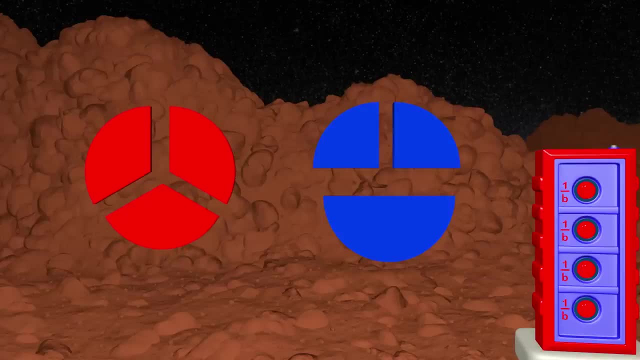 To be a fraction, you must have all equal parts. The blue circle on the right is not divided equally, so it cannot be a fraction. We also need to review how a fraction is written. The fraction we see is 1 over 3, or one-third. 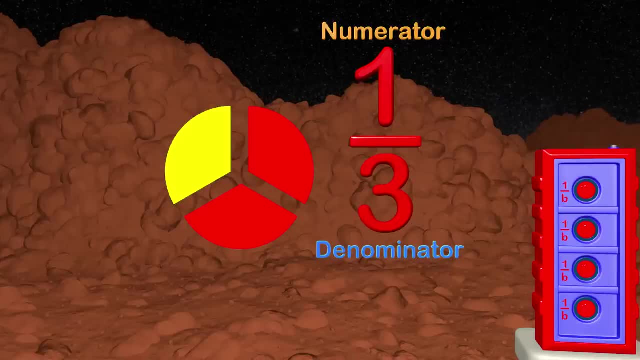 The top number is called the numerator and the bottom number is called the denominator. The numerator is a part of the whole circle. The numerator is 1 because there is one yellow part of the whole circle. The denominator is a part of the whole circle. The numerator: 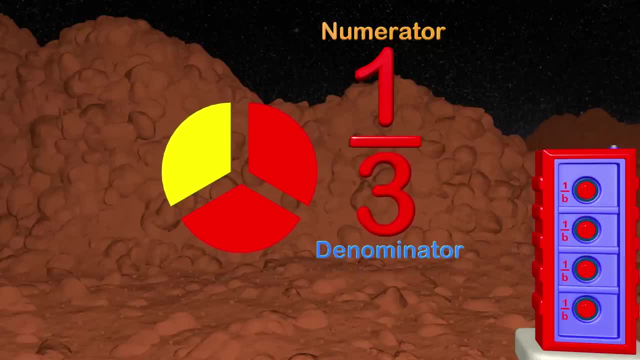 The denominator is the number on the bottom that shows all the parts in the entire circle. Because the entire circle is made of 3 parts, the denominator is 3.. This fraction is 1 over 3, also called 1 third. Now that we have this out of the way, let's move on to recharge my spaceship.